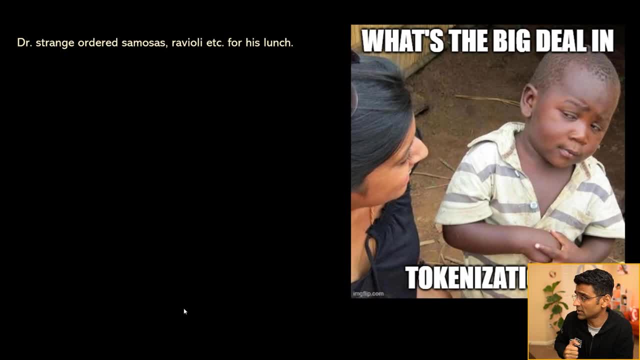 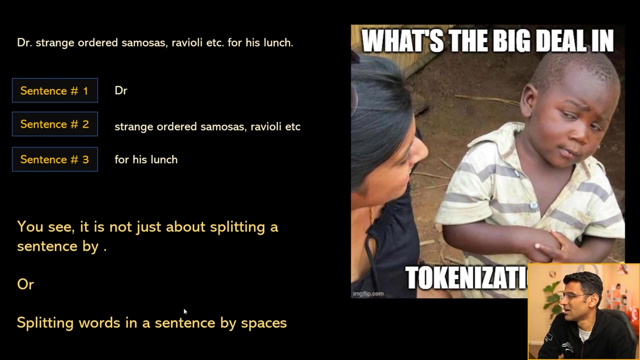 we need a library. well, consider this statement. if you are doing sentence tokenization for this. for sentence tokenization you might use dot. dot means the sentence is ended. if you use that simple rule here, you will end up creating three sentences for a sentence which is just one sentence. okay, so you can't use simple. 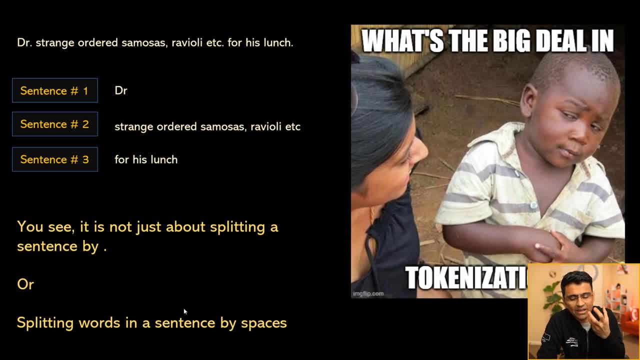 rules for this tokenization. you need the language understanding. you need to define spatial rules that dr, doctor, dr dot is not the end of the statement. also, if you have end dot, y, dot, it's not. dot doesn't mean end of the statement. you need language specific rules here. 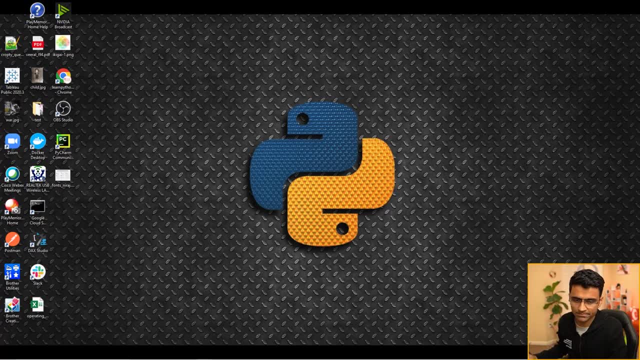 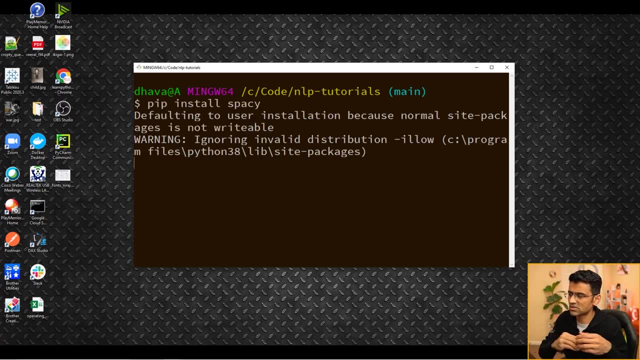 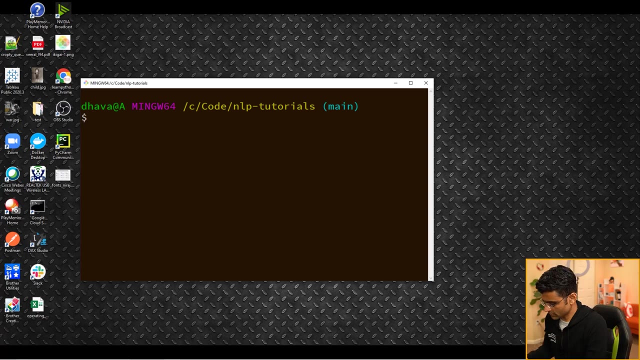 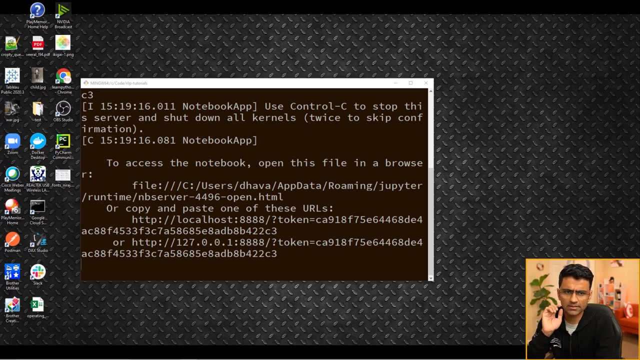 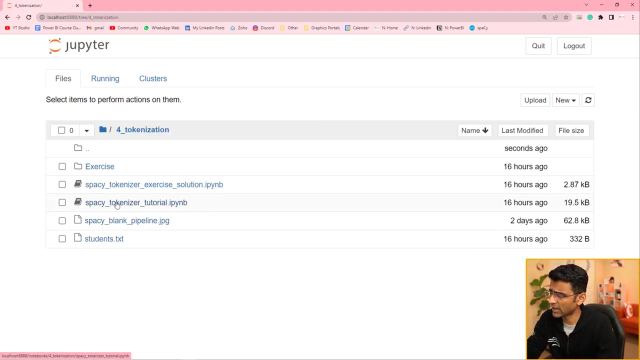 so what we will do now is, if you have not installed already, just do pip, install spacey and that will install the spacey library on your computer. i already have it installed. to launch a jupyter notebook. you can run jupyter notebook command and whatever directory you run that command in, it will show all the files there. so i, i'm, i will, i. 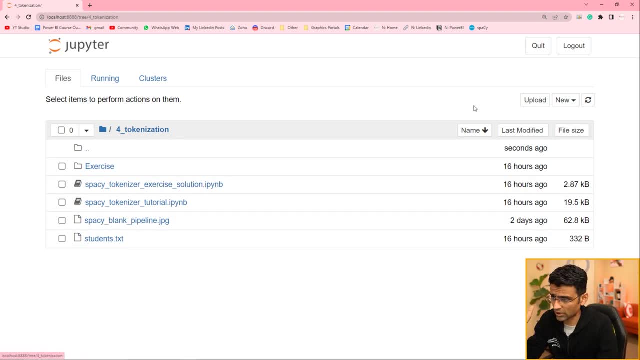 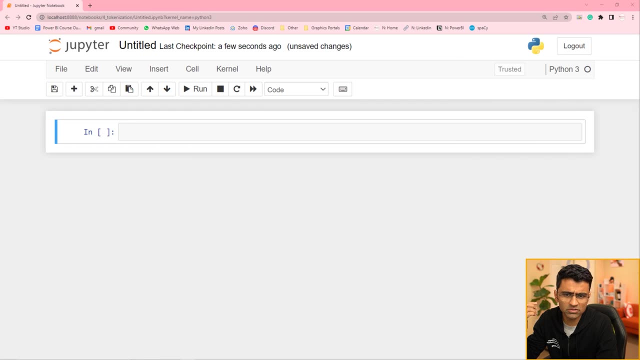 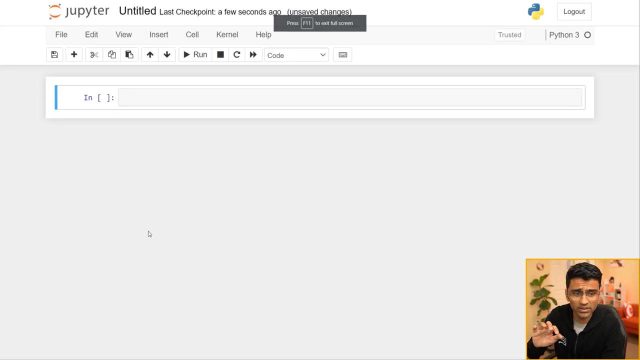 have created this spacey tokenization directory already, so you can create whatever directory you want and just say python3, right? so i'll just move everything else aside and i will do f11 to bring this in a full screen mode, and then i will just create this in a full screen mode and then i will. 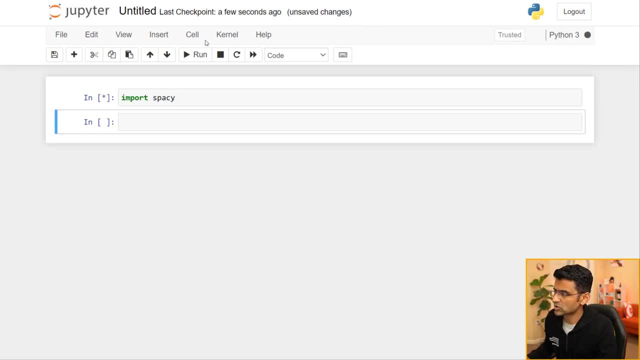 import specie, so that will import the library, then i will create a language object. so in specie you can create language object in multiple ways. one way is you can just say specie, dot, blank en en stands for english. okay, now, that creates. so just simplistically, think about nlp. 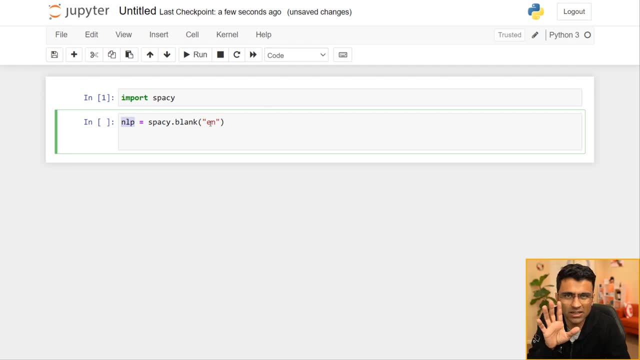 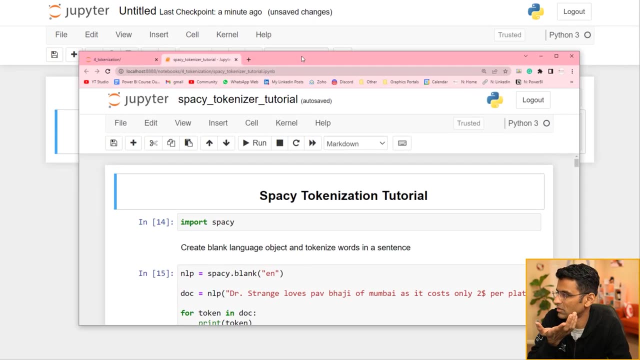 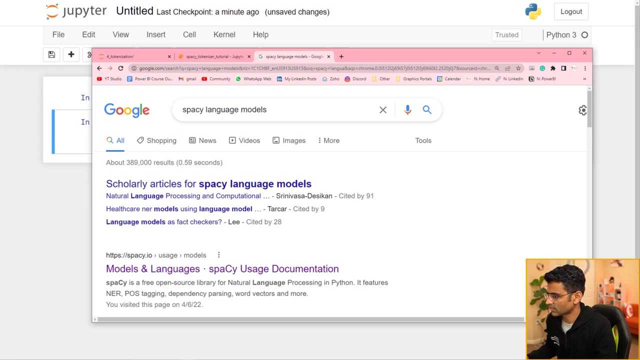 as an object which has english understanding. it understands english language a little bit. if you say de, it will be for german language. now i, how do i know? like, whether it's de or en. like that's like magic, so you can say specie language models and it will show you. 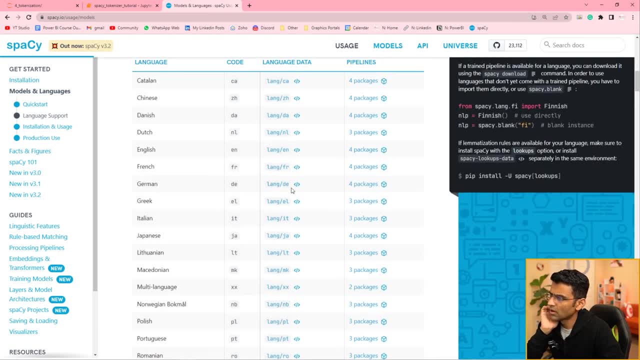 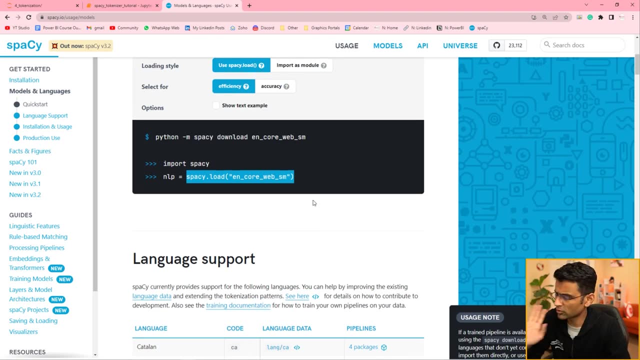 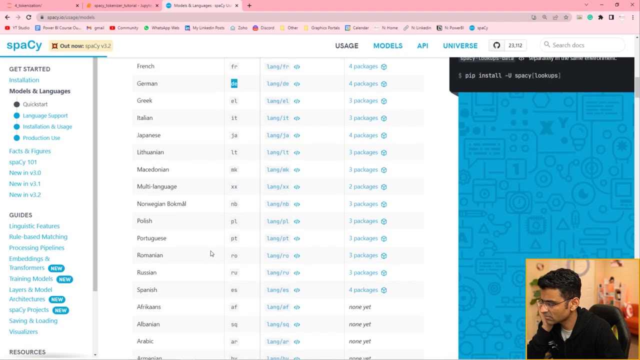 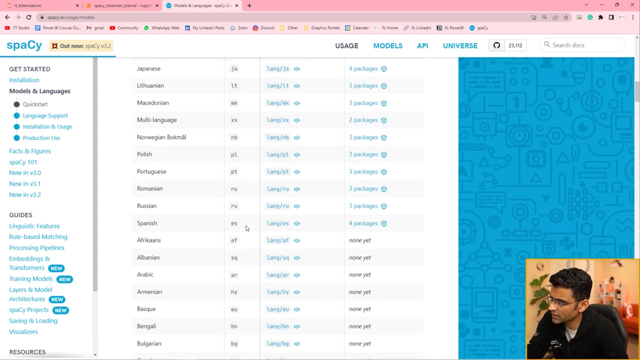 all the language models. you have right, so we will do something like this later on. this is more like a trained language pipeline, so don't worry about this. but see, english is en france, french is fr, german is de- okay, hindi is hi. so whatever language you are dealing with, first create the blank component there. 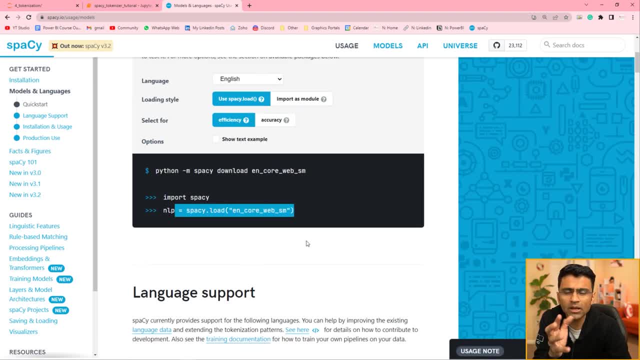 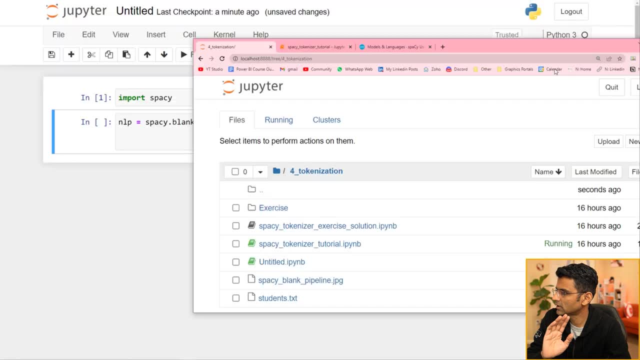 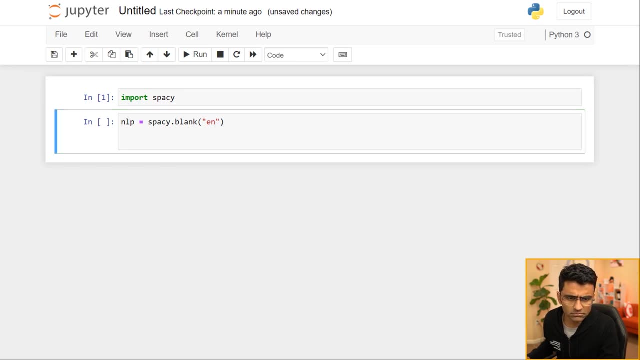 is another way, which is creating a pre trained like pipeline. we'll look into it in a later videos. so this is how you create a blank component. so this is how you create a blank component. so this is how you create a blank component- English language component- and then you will create a document. so document is. 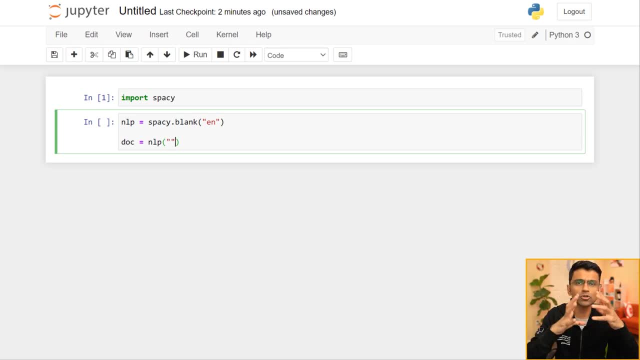 equal to NLP something here you provide your text. so whatever text analysis you are doing, it could be a paragraph, it could be a multi-page document. you need to provide a text here and the text I'm going to provide is dr strains visit in Mumbai. he loved power body so much and I'm doing some text analysis on dr. 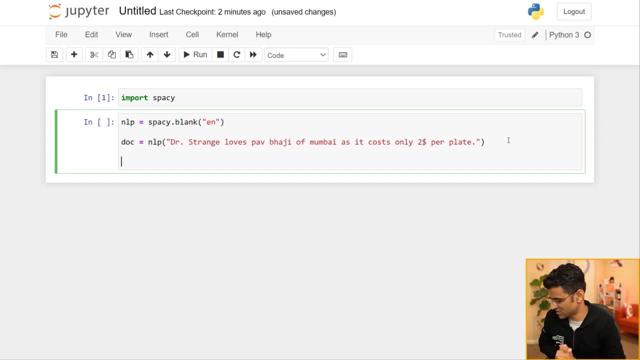 strains, beautiful journey into Mumbai, and poverty. so when you do this by default, what this will do is it will give you a text that you want to provide, a text. so what you can do is by doing this, see, you can do for token in doc, print open and when you hit that it has already done word tokenization. it is so. 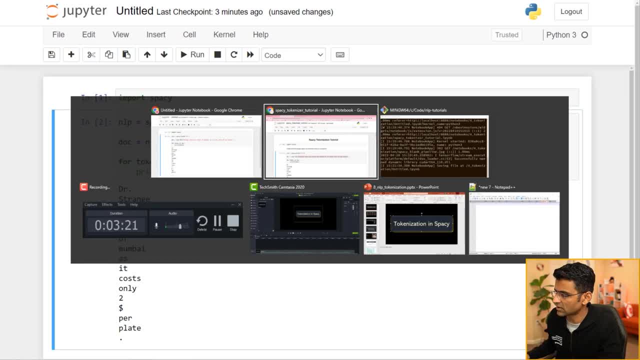 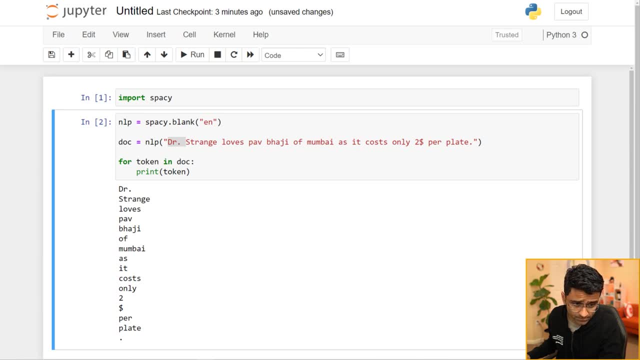 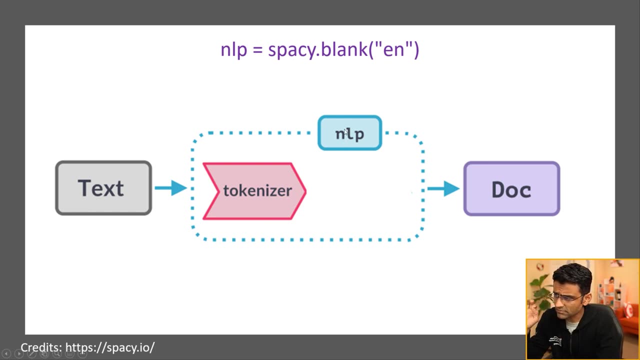 easy, plain Python code, very intuitive to understand. and, if I go back to my presentation, what it is doing in reality is this: so when I say spacey dot blank, I created an LP component around the text that I had by default, it gives you a tokenizer word tokenizer. so when you 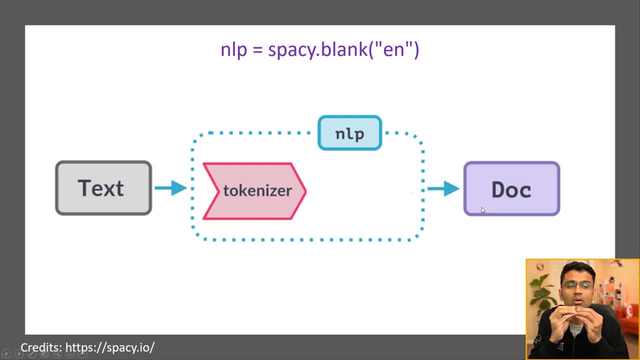 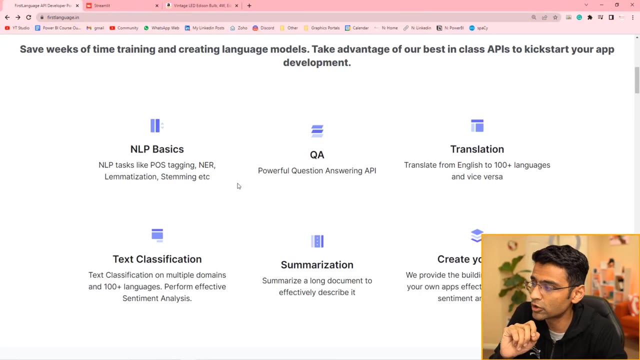 feed text into it, you get doc document. doc document already knows about tokens, so it has like token 1, token 2, token 3 and so on. I want to take a moment and talk about first language dot, in which makes building an LP application easier for you. you can perform various NLP tasks which are shown here via this. 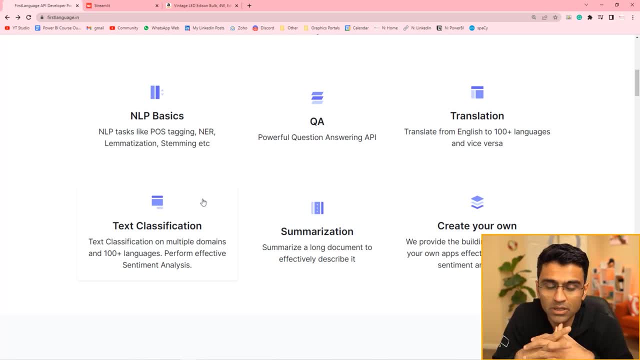 platform. if you're using a spacey type of library, you download it. you run your code locally. if you are training a heavy model, you need higher compute resources, such as GPUs, whereas here everything is in cloud. you just make an HTTP call. things run on the cloud. you don't need a local machine with lot of compute. 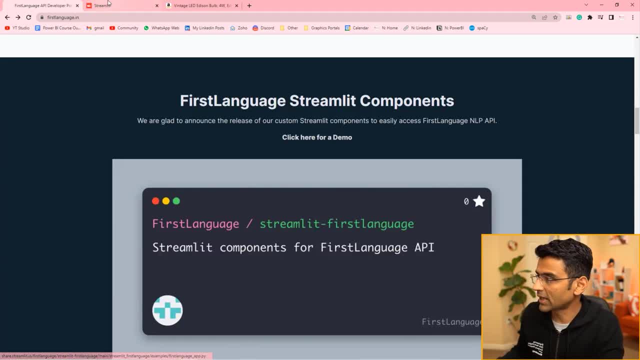 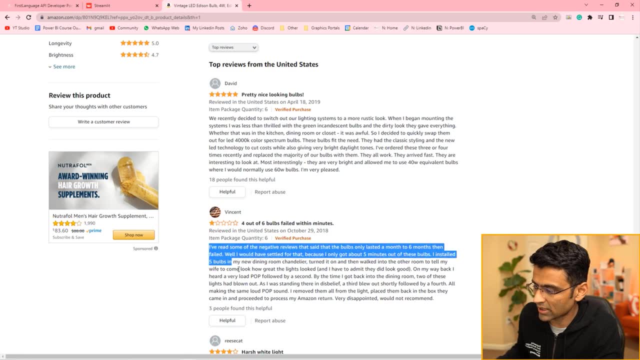 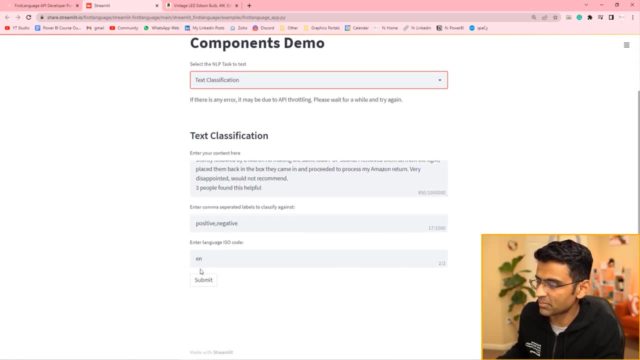 resources. there is a demo which you can see by clicking on this link and I have bought this bulb recently and you see there is a negative review on Amazon and when I copy paste this here and I select text classification and when I say submit, it immediately classifies that as negative. 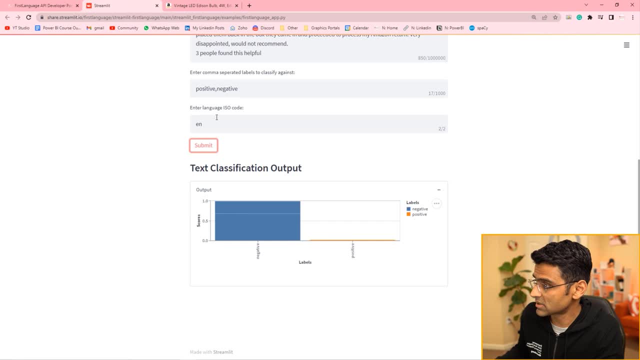 and if I have a positive review, I just copy paste it here, and if I submit it, it will classify this as a positive. it's pretty powerful, so it will classify the positive. and then it will classify it in the negative, so it will classify the positive. you see, it's pretty powerful, so it. 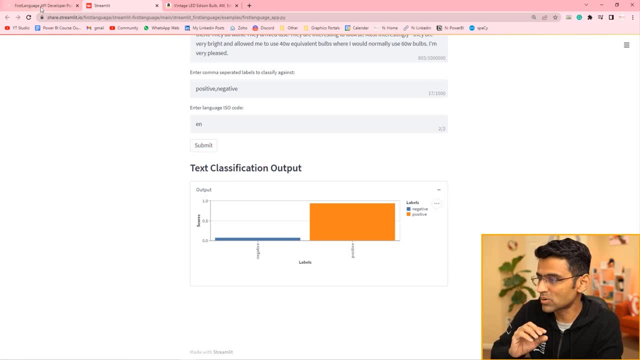 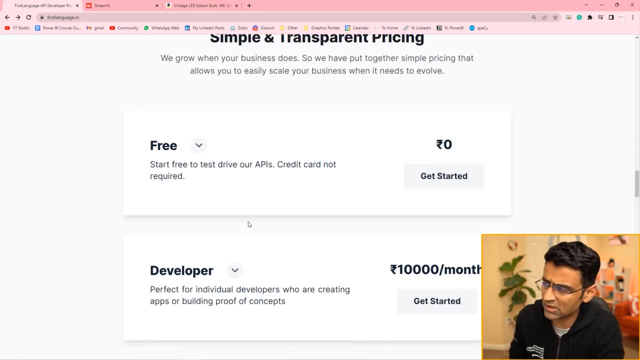 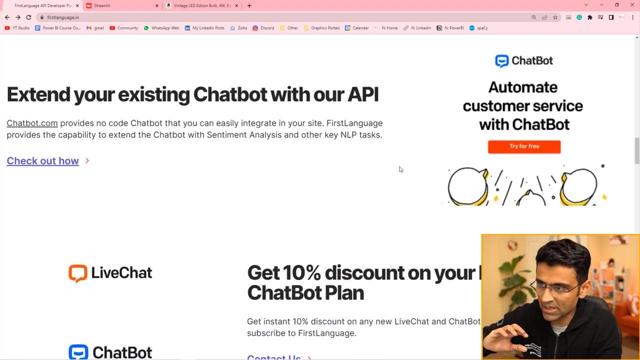 It makes things much easier for you. You don't need to have like too much like detailed knowledge. You can just call APIs and get things done quickly for yourself. The free tier is something you can try today. You can just sign in and you can get an API access. 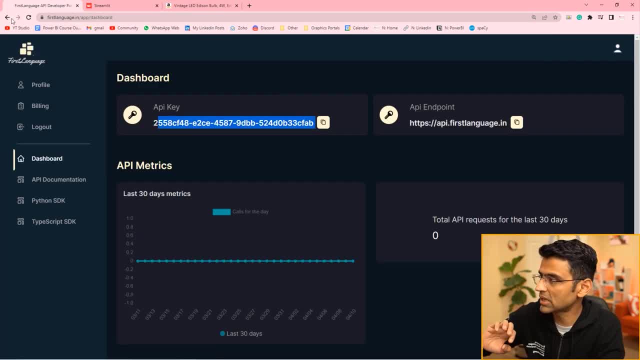 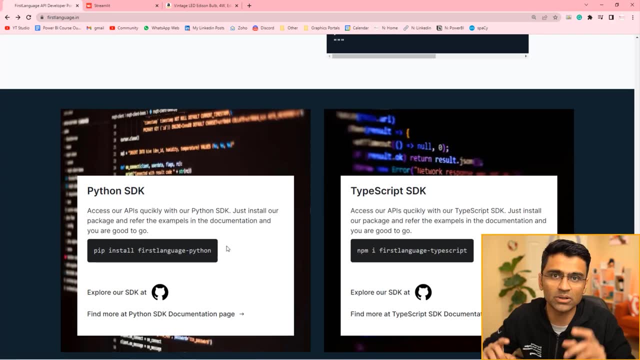 Once you sign in, if you go to dashboard, you'll get your own API key and you can use that API key to make the calls. They have SDKs available both in Python and TypeScript. Go check it out. The link is in video description below. 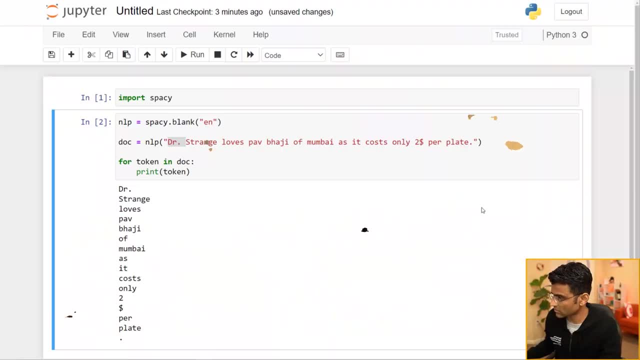 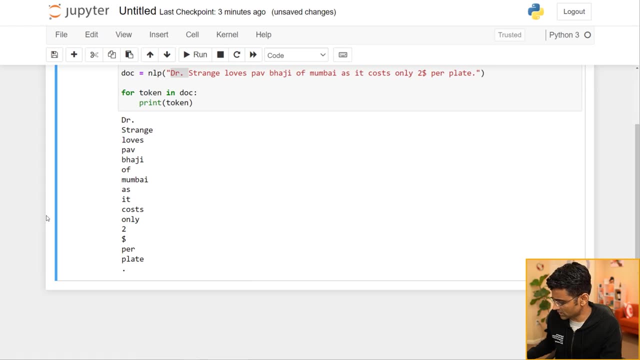 And thanks firstlanguagein for sponsoring this video. So that part, I think, is clear. Now these tokens: either you run a for loop or, if you like, Python list style of index. you can do this. also You can do log0sdrlog0sdr. 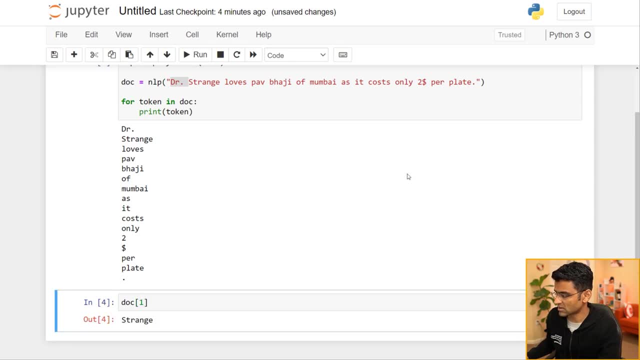 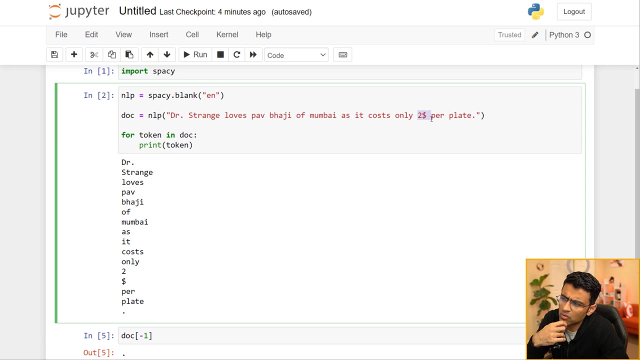 So you can use general, like Python, list, like index operation to retrieve all these tokens And you realize, if I have two dollars, the English model that we created it understands that this is a currency. Therefore it will split two and dollar into two. 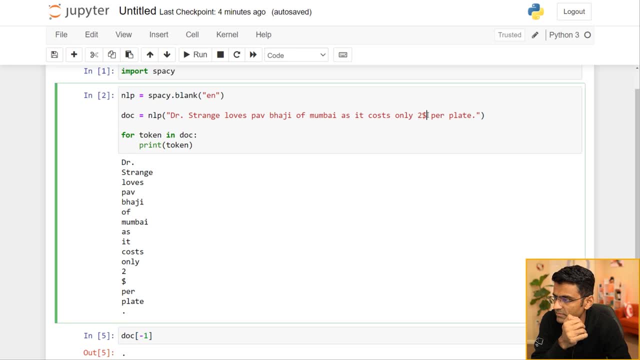 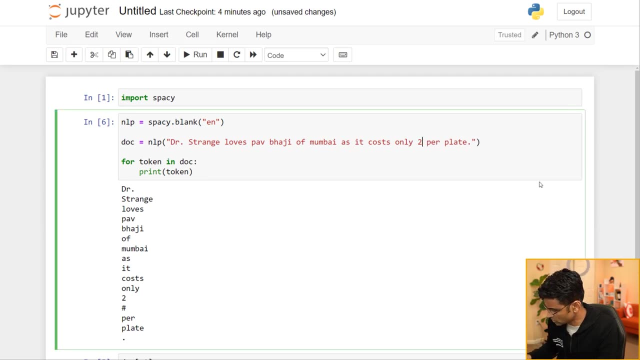 Two different tokens. So let's try this: If I do this hash, I think hash also is splitting it into different tokens, So it probably OK. so currency, the punctuation, it will split them into different tokens. If I was using just splitting by the words, then it won't be sufficient. 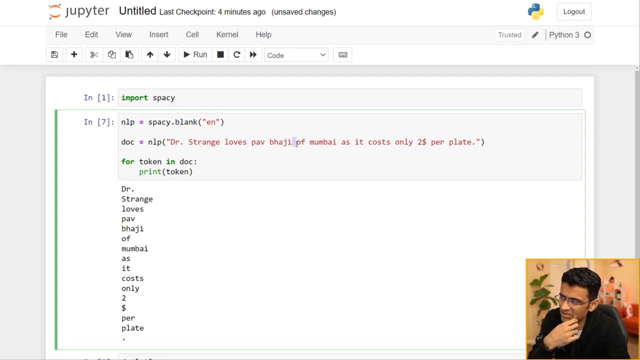 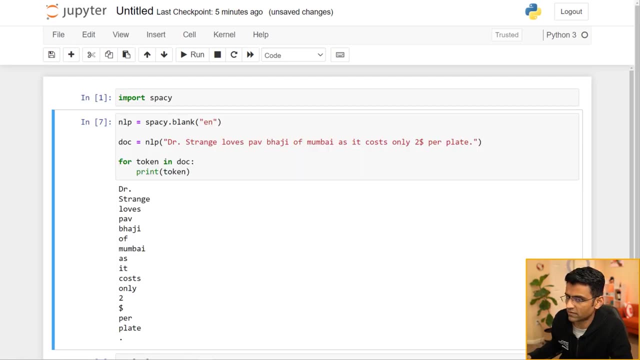 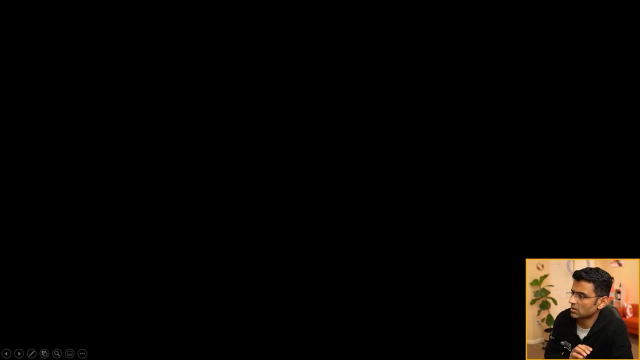 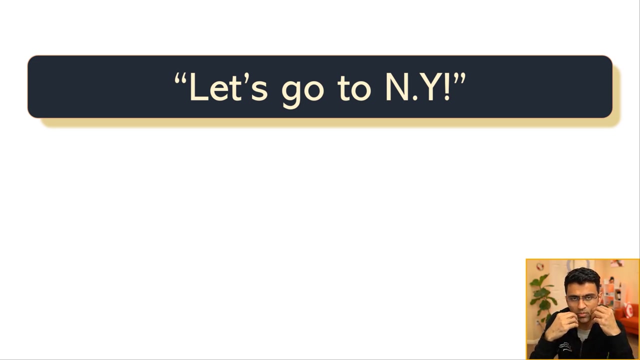 Correct And it doesn't. it's not smart enough to detect the language And let me explain the rules of the tokenization, So I got this image, Not this image. I got this image, by the way, from spaCy documentation. 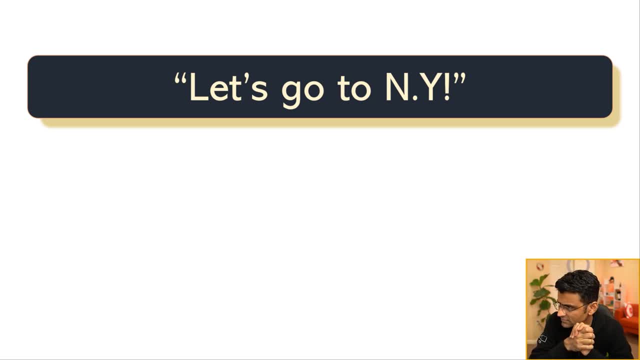 So thanks for that. But let's say: you have this sentence, Let's go to NY. The sentence has double quotes. OK, So if I just use split By spaCy, I will get these, these words, and these are not my true tokens. OK, 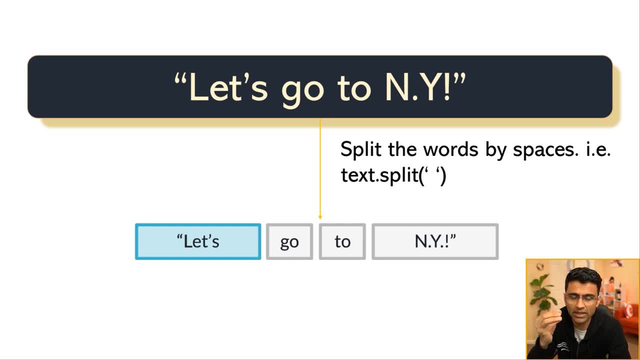 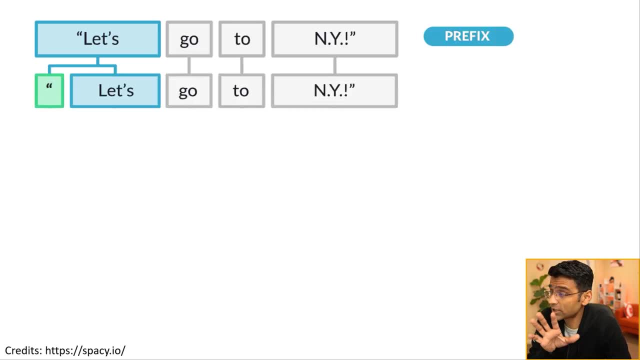 That's when spaCy tokenizer tokenizer come in place and it will do some additional processing. OK, what kind of processing? Well, this: It will first split by prefix. So any prefix you have code, that's a separate token- It will split. 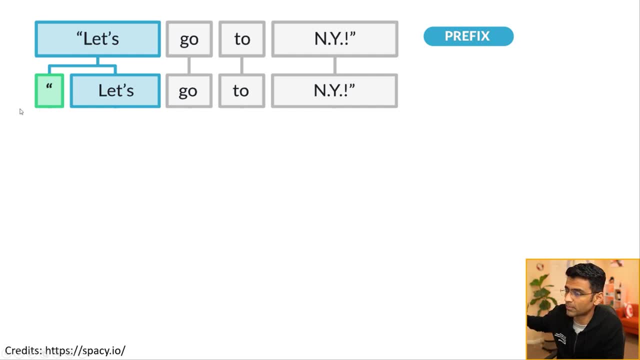 See you green box. It just splits that as a separate token. It could be dollar sign bracket that are. there are some characters it considers as prefixes and it will split them. Then it looks at exceptions such as: let's see apostrophe s. 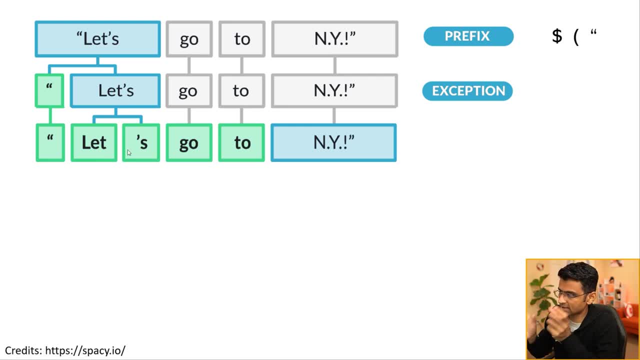 That is also a separate token. And when you do that this kind of, when you do splitting into this kind of individual component, I will show in a later videos that this is very beneficial for doing the language analysis, for building the NLP application. 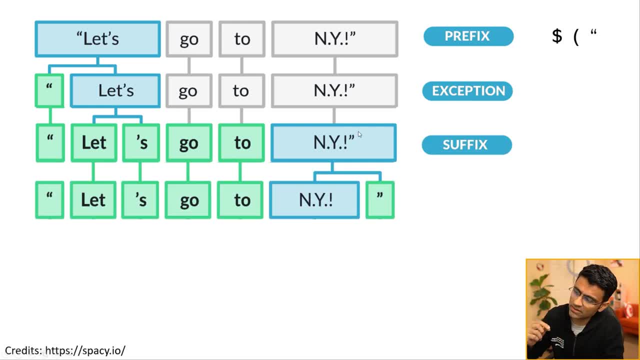 Then you do suffix, right, The way we did prefix. there is a double quote at the end, So that's my suffix. Then you have one. OK, suffixes could be whatever km is kilometer, It could be bracket, explanation, exclamation mark, quote, etc. 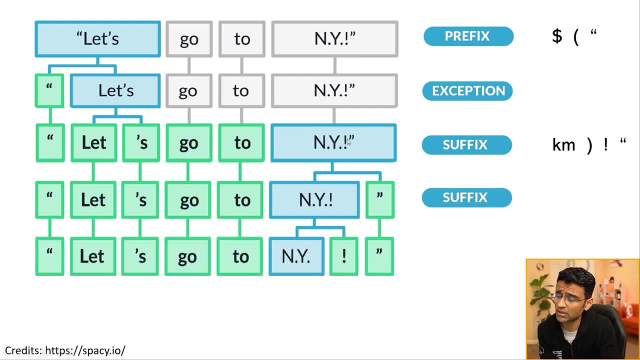 Then, Then another suffix would be the excellent exclamation mark after and why? to split that, Then one more exception would be. I think Yeah, So the exception is split. OK. so suffix was this and the exception was this. So now you split. 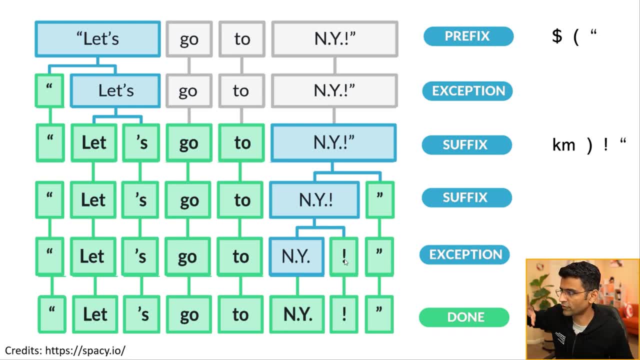 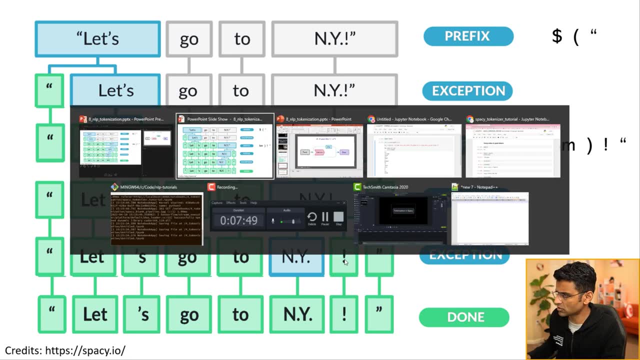 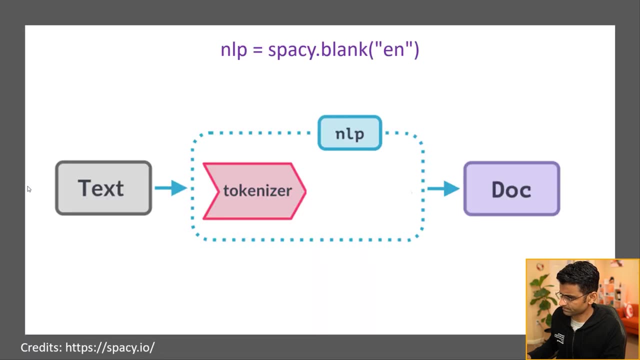 Now your tokenization is complete. So if you feed this into spaces tokenizer, let's go to and why you will get these kind of tokens. You want to try that, by the way, let's. how about we try that? That would be nice. 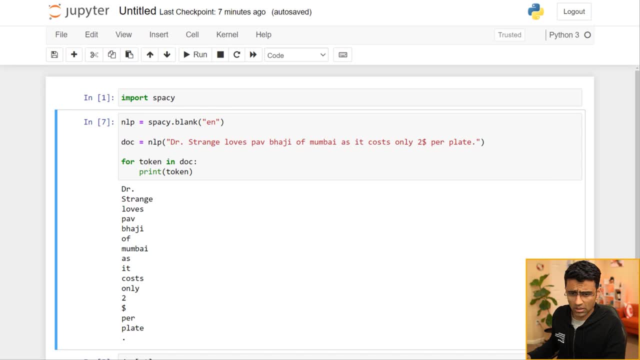 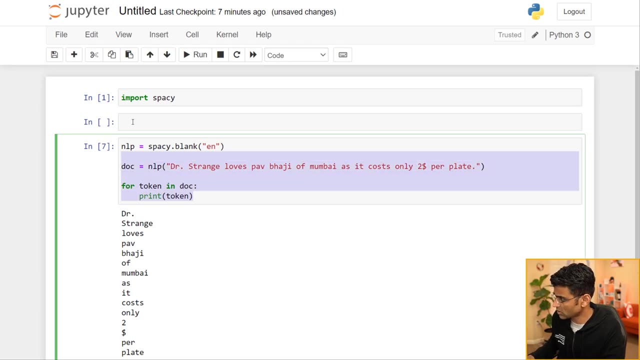 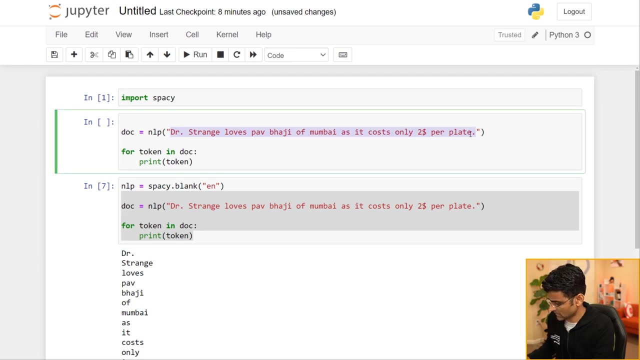 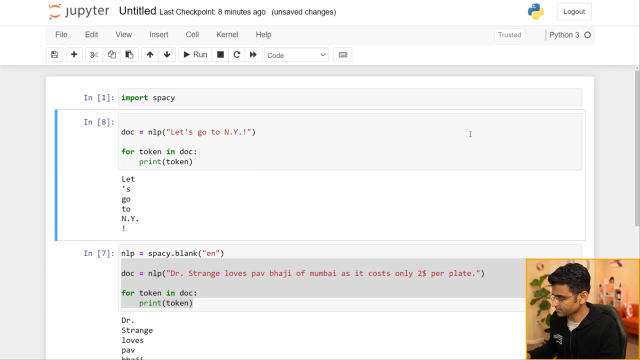 So instead of whatever Dr Strange I can, I'll just do it at the top, Because I want my Dr Strange to stay here. So I will say: let's go to and why dot? see? let's go to and dot. why dot? exclamation mark. 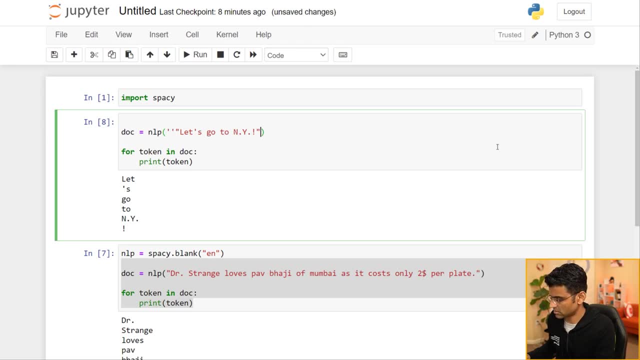 See, and actually we need like single quote, Because I have double quote as part of the sentence itself. OK, so, OK, there is a single quote also, So I will use three quotes. actually, I will use three quotes, by the way. 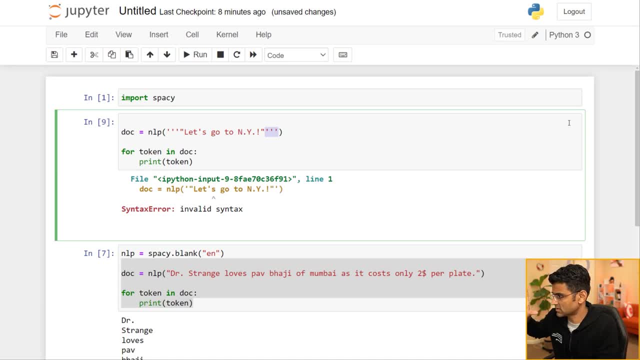 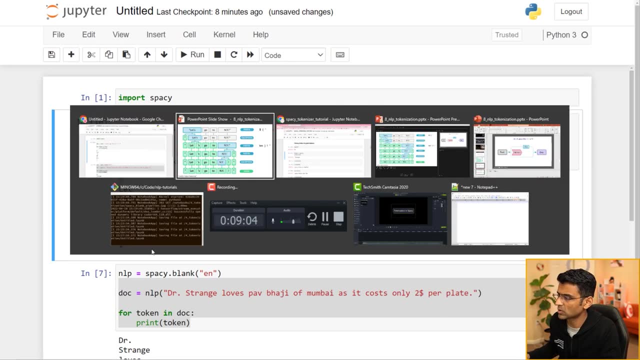 So you know, I take three quotes is like a whole sentence, And since I have a single quote here, that's why I'm using this. Anyway. But see, this is one token. See double quote. Let's see. 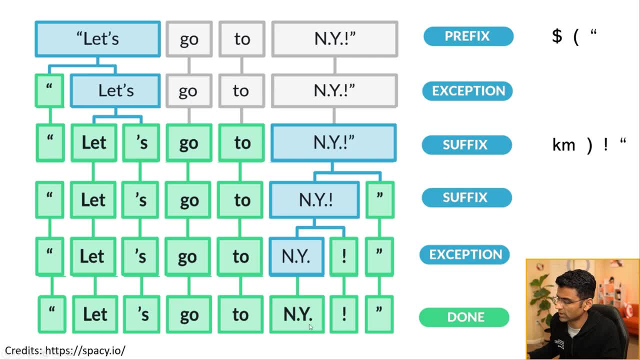 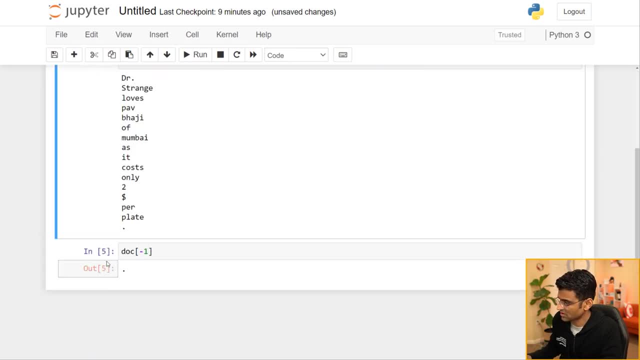 Let's Yes, Then go to go to. and why? So it works. I just wanted to show that I'm not bluffing. OK, it works. And then we looked at the index operator. Now let's look at the type of this object. 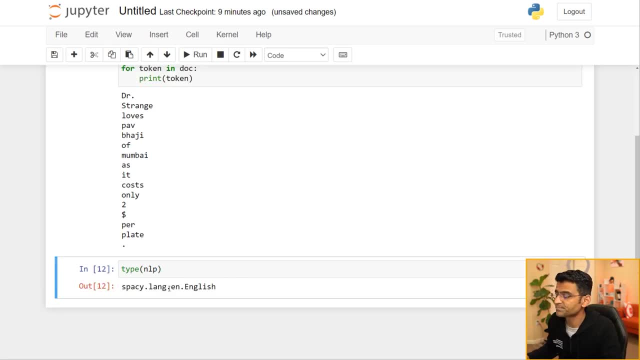 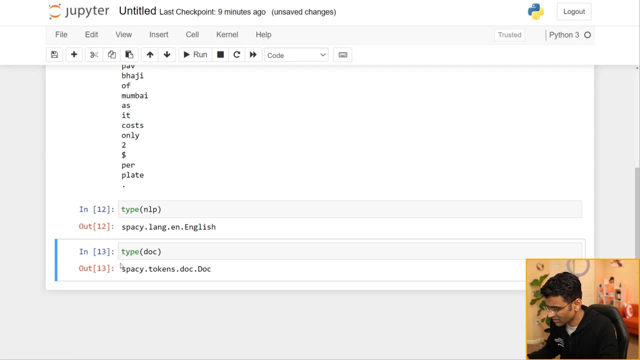 See NLP. I say: right, it's, it's an object of English language. Similarly, if you do doc, that's an object of a doc. Come on, Isn't that? clear Token is an object of token. There is a span object, by the way. 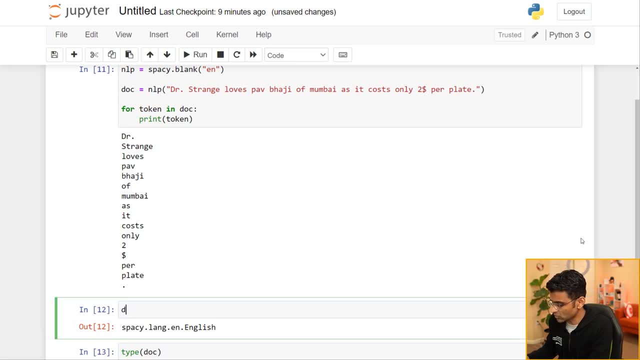 So I have all these things right. If I do doc, see, if I do doc one, whatever, it gives me one string. But if I do something like one to five. you have studied this slice indexes in Python. Correct, It gives you a slice. 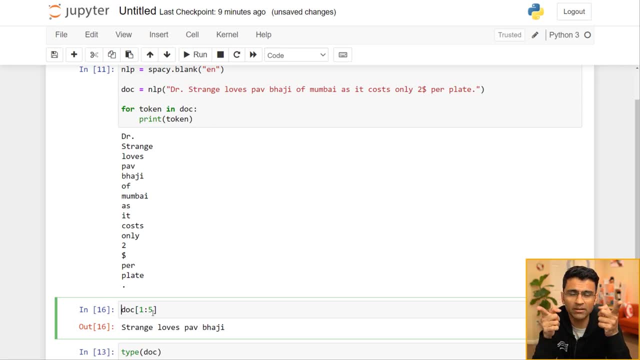 Similarly in NLP. Also, If you want a span from a sentence, you want certain span. Span means a sub string from that string And this object is of type span. So if you do type span- and you will see in the later video how this is useful- 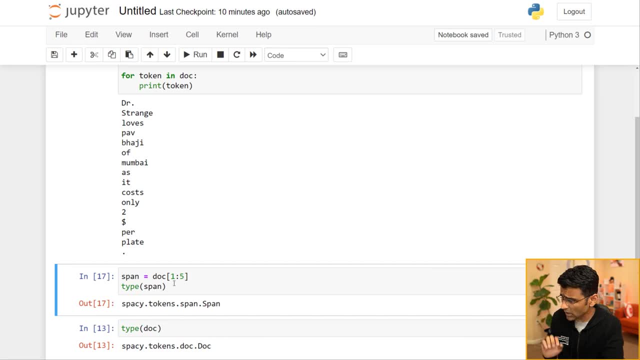 You get an object of span, The OK. so let me just clean all this up. Let me come up with a different, Different sentence. OK, so Tony and Peter are friends, They have a mentor, mentor relationship And Tony gave $2 to Peter so that Peter can buy the car. 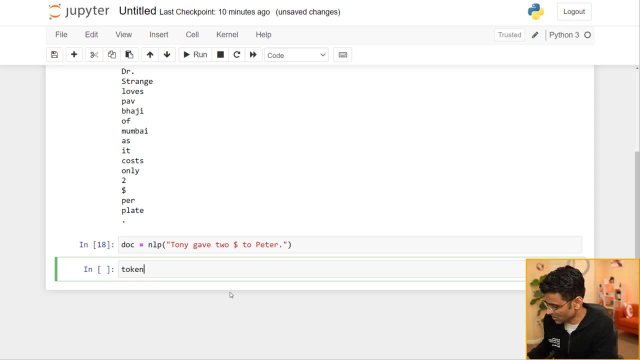 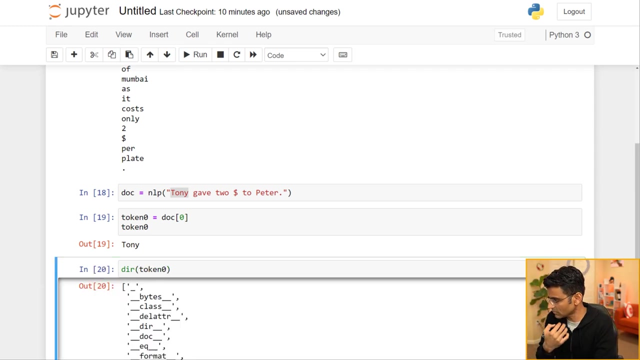 OK, Just kidding. So token zero, is this correct? And that token zero would be what, Tony? Now, this has certain attributes. So if you do dir in Python General rule, If you do dir on any Python variable, you get all the methods and everything of that. 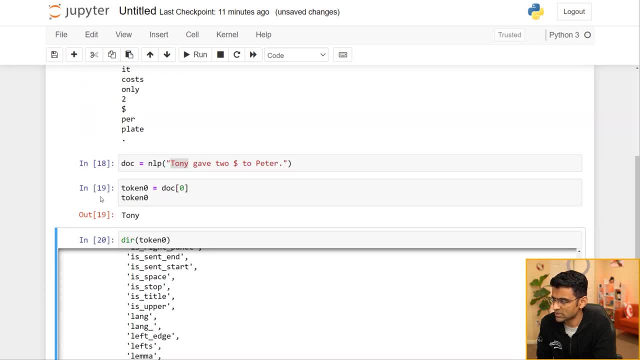 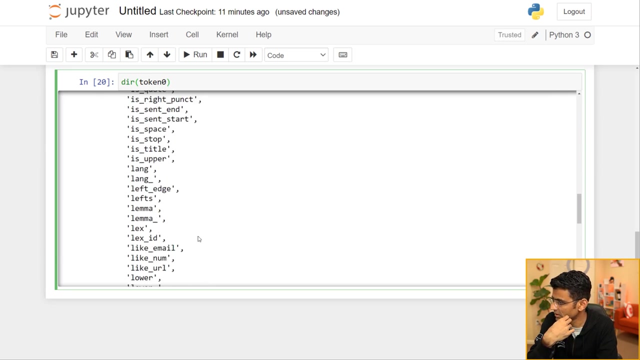 class. So my class of token zero is token correct. If you do type of token zero, it's an object of class token And that class token has all these methods. See all this. See is bracket is currency, is digit Each stop. 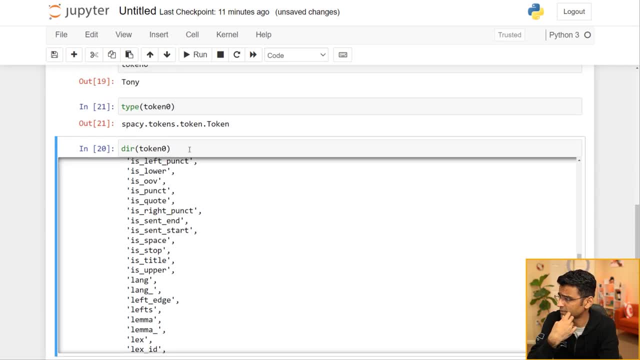 So let's try to use some of these methods. So I will first use token Zero. dot is And if you hit tab it shows all the matters as a help. So I will say: is up, It says true, Because it is. 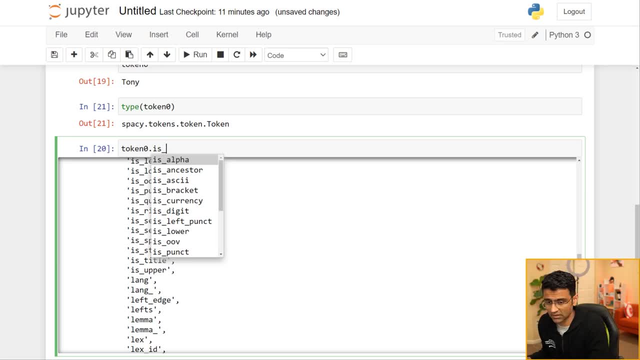 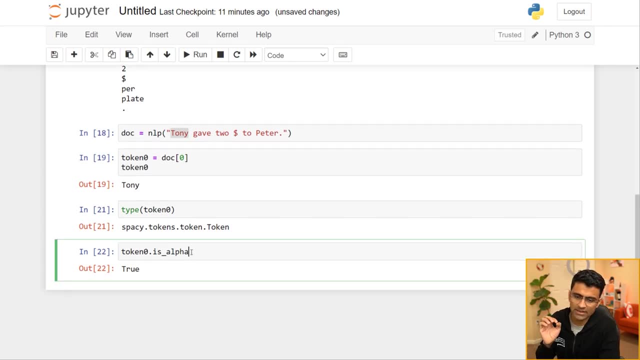 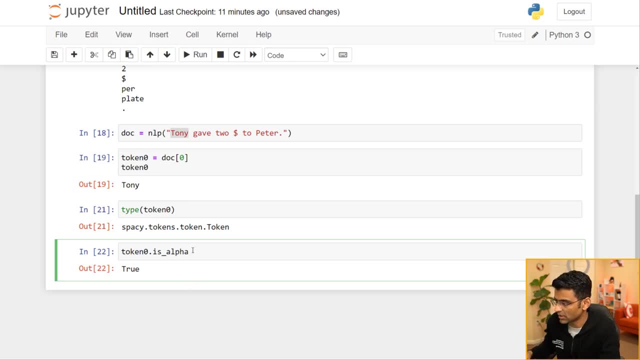 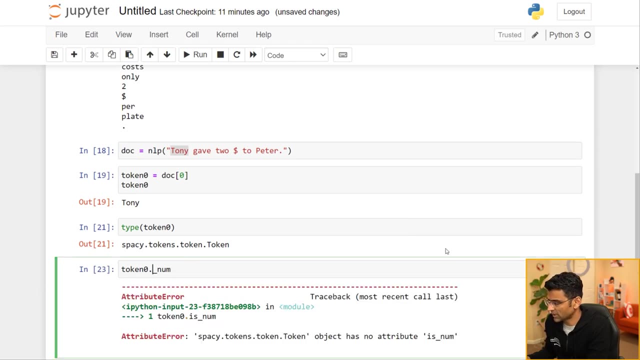 It's a word. It's a word. It's just alphabetic Is a word, It's a word. Basically it's not a number. if I do, is none. Actually, the method is like none. He says for its not a number. 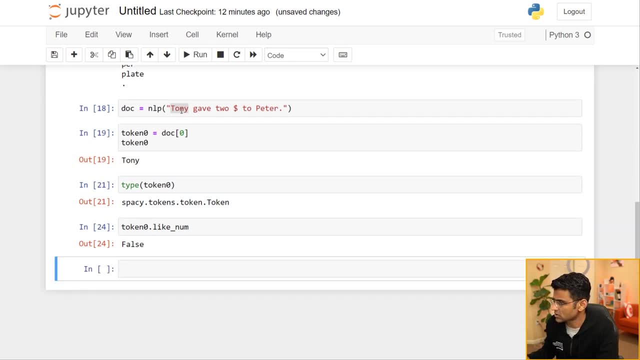 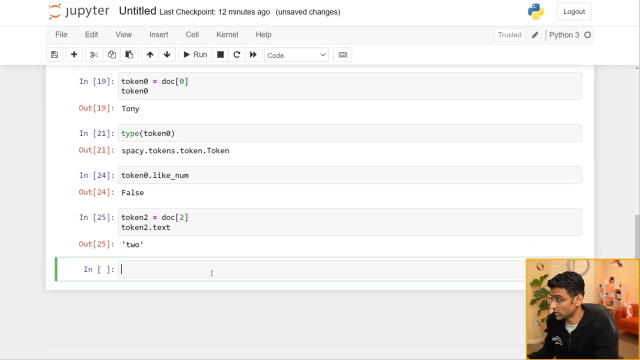 Correct. But but let's look at this. So zero, one and two. Okay, so Two is equal to two. Let's print- and by the way, you can use token two, doc text Also- that discutable you the text. so this token two is the word two. now, if you call this method, tell me what's gonna happen. 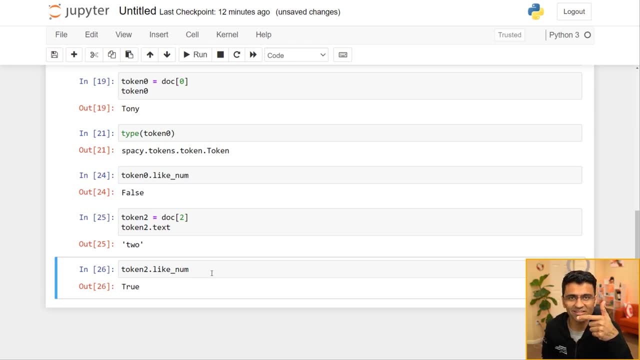 any guess. see, this is smart. it knows tw2 is a number, it is like a number, and it tells you that that is true. what is token three? okay, let's try token three. token three is that dollar sign and luckily we have a method called is: ah, is currency. it says: is currency true. 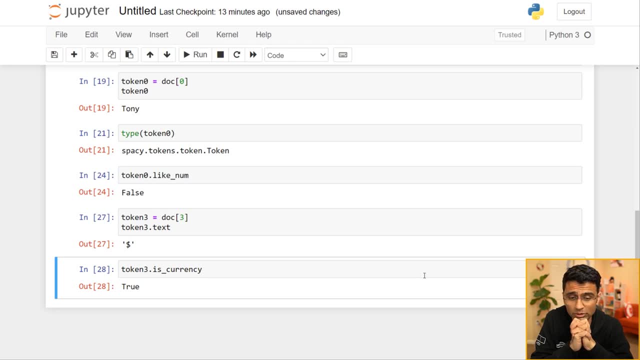 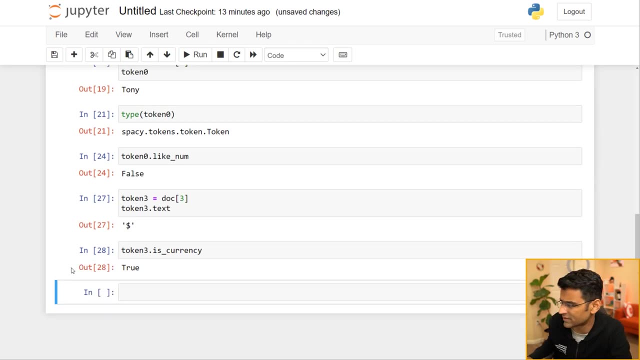 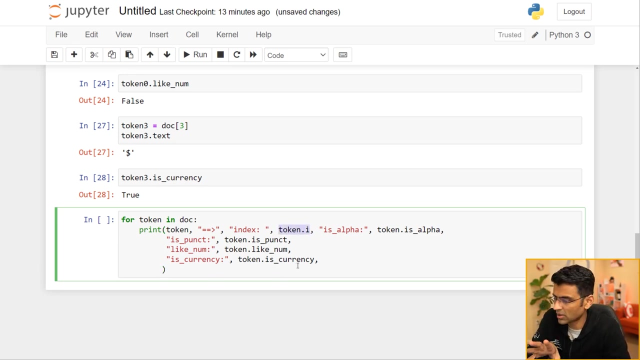 hmm, now this can be pretty powerful. okay, so i can show you a use case, but let me first print couple of just few of these attributes. so i'm running a full loop. i'm printing a token. token has an index which, which is called dot i, is alpha, is something we saw is punctuation. 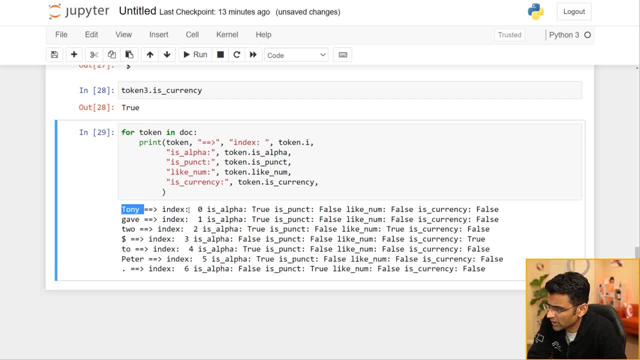 like number, like like currency. see for tony, it will say it's not like currency, it's not like number. but when you have dollar it is saying it is currency, it is not a number. but when you have two it says like number is true. so these 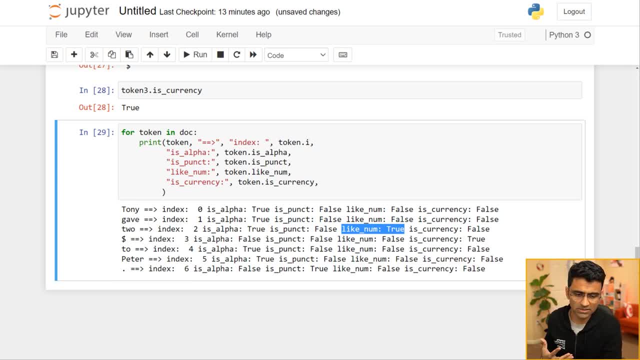 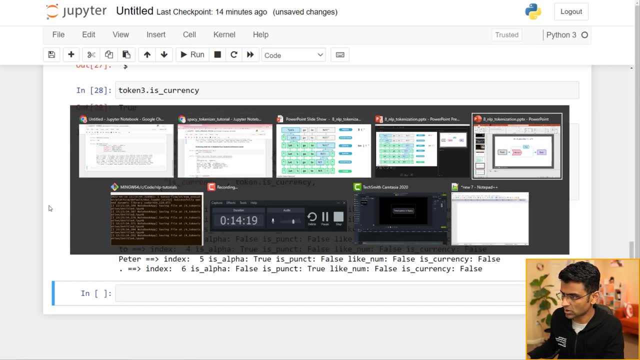 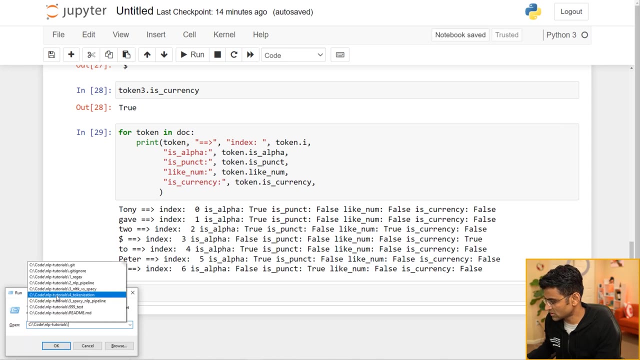 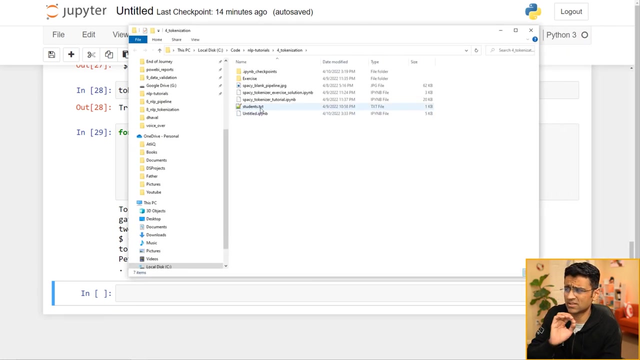 these attributes can be pretty powerful in doing your text analysis. now i'm going to um quickly show you a file, so let me go here. so i am in my c code and the tutorial series now in the date vr file where i'm running- uh sorry, directory which has a file called. 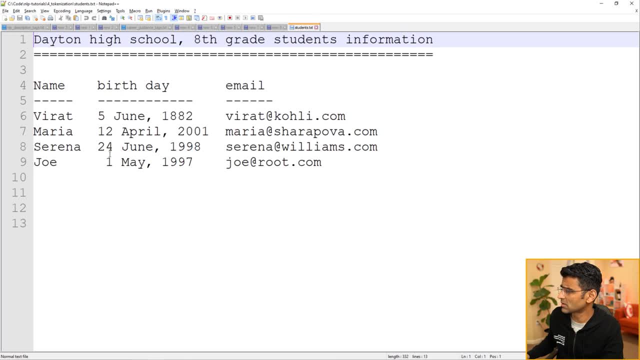 studenttxt. okay, what is there in this file? i'm curious. ah, it has some student information. see, in my class i have pretty talented, some talented students. you know they come to my class too to learn python, by the way- all the students, they'll get pretty good in python. 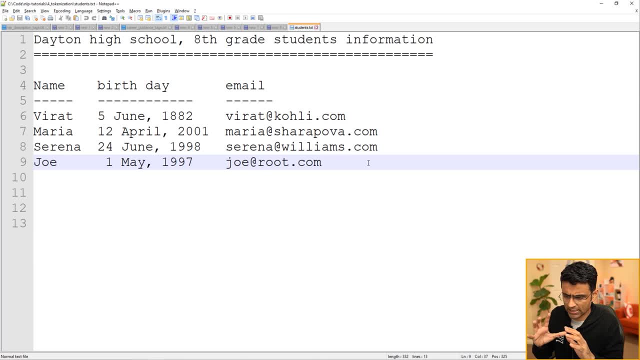 and let's say i'm a teacher and i have this text file ofuzu now so i can spell just like we seen in latin of all the students. and let's say tomorrow is gonna snow, so I want to declare a holiday, so I want to send an email to all the students saying that: 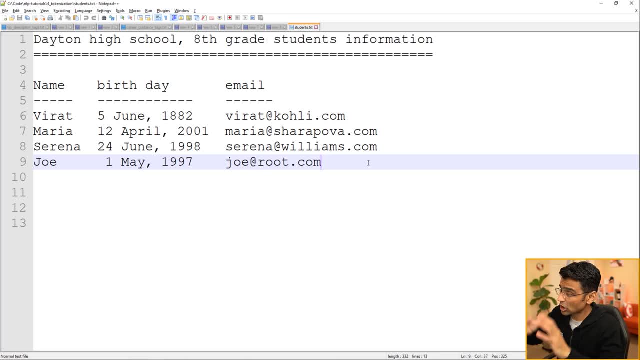 tomorrow is holiday, hurray, enjoy from this text file. I am showing you a simple text file, but this text file can be very big. how do I extract all the emails? all I want to do is, from this text file, I want to extract all the emails I can use. 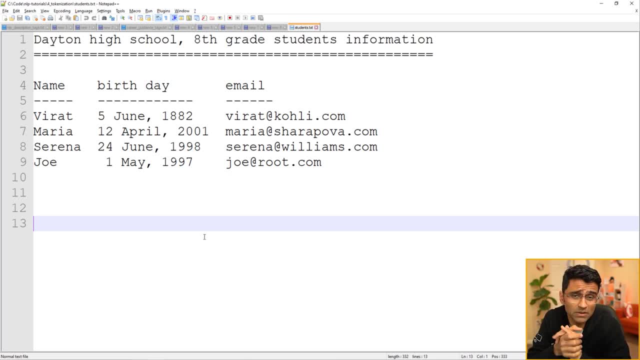 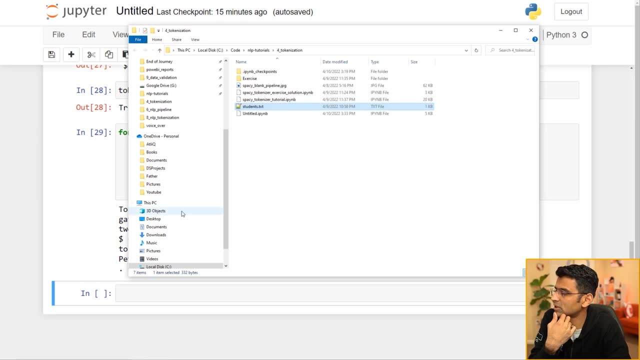 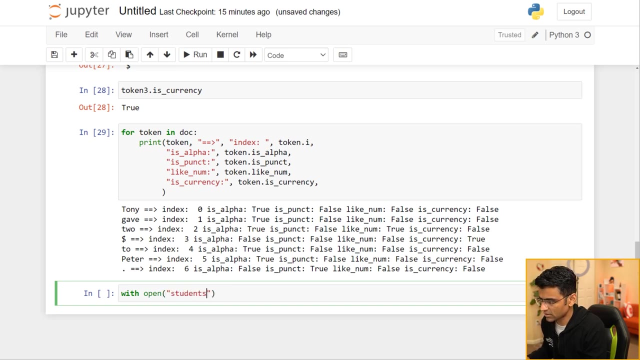 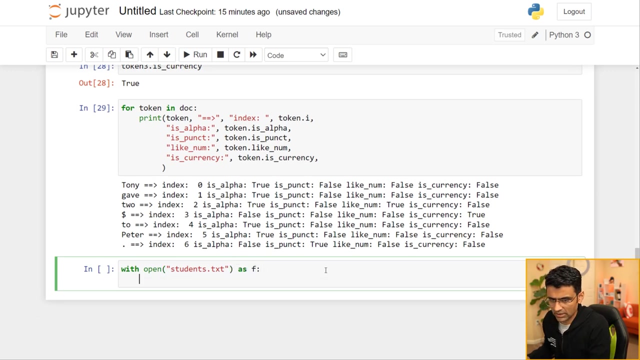 regex. you know regular expression. there is something we have seen before, but on this occasion I find like spaCy can be even more convenient than regex. so let's try this. let's first read this file in Python, so you all know how to read the file in Python when you do freadlines. 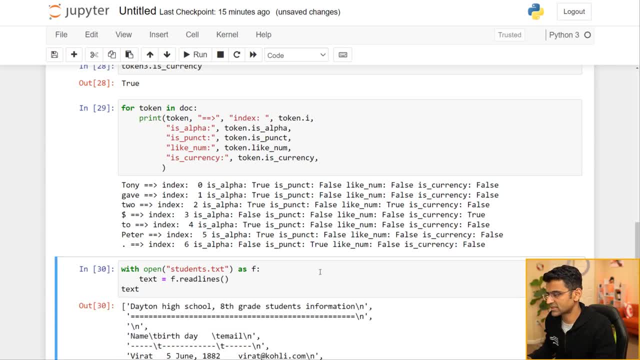 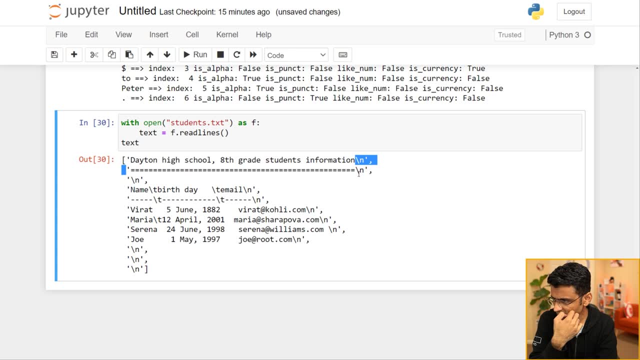 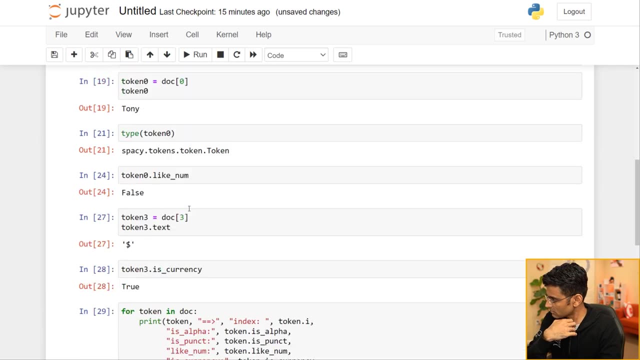 it will read all the lines in a text file as a text as as an array. so text is an array of all the lines. you know what slash n is right for the new line? now spaCy takes single text, so I will convert this array into single big blurb. 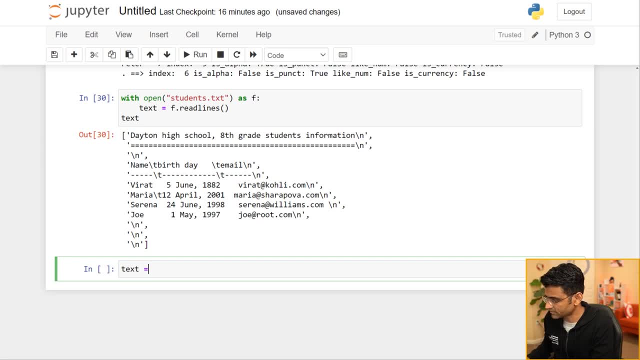 of text. okay, and the way to do that would be. so I'm separating everything by space and I'm saying this. so what this will do is text is an array, right, list. it will join all the elements by list and it will use space as a delimiter in between the list element when they join. it will use space. 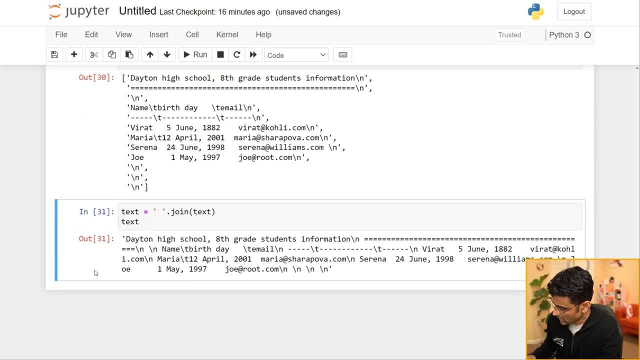 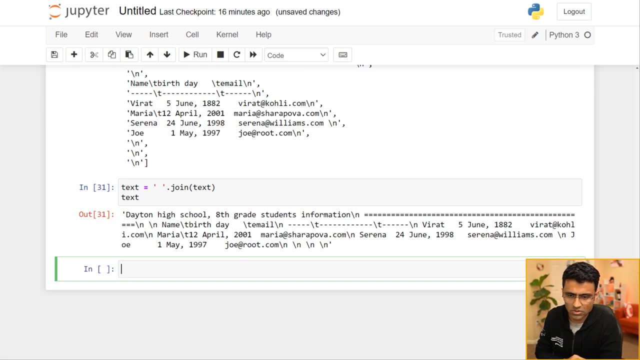 in between. great, so it's a one single sentence. now I want to grab all the email, so I will first create a document element from this text and then I will say: for token in doc, if token dot, if token is like email, then do something I can print. but I don't want to print, I want to. 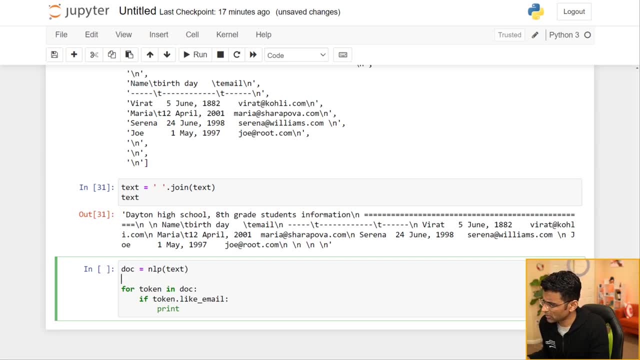 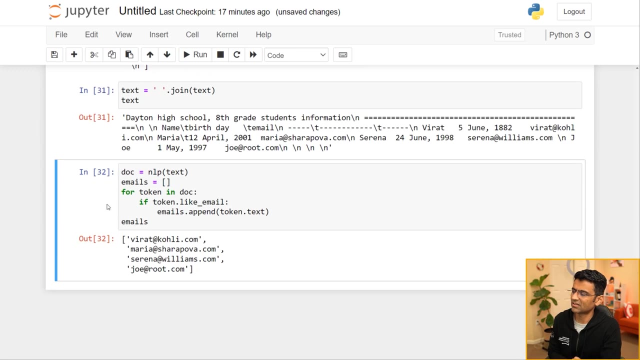 I want to grab maybe all the emails in emails array like a list, and the list has this method called append token dot text, and when I do that I get the emails of all my obedient and intelligent students. this is one simple use case. you have other methods too, like. 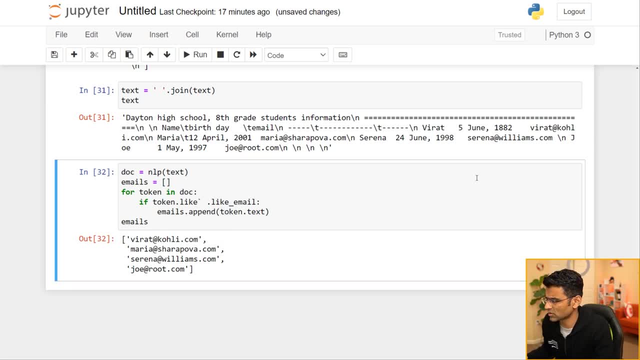 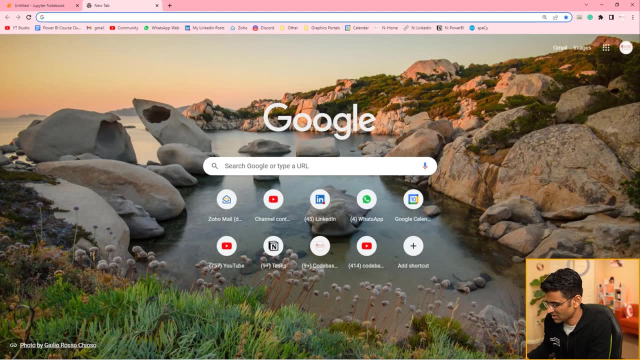 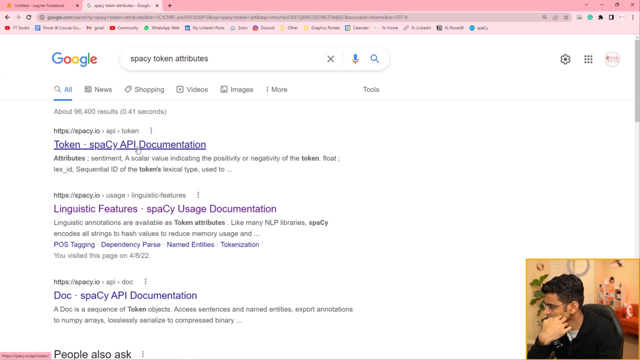 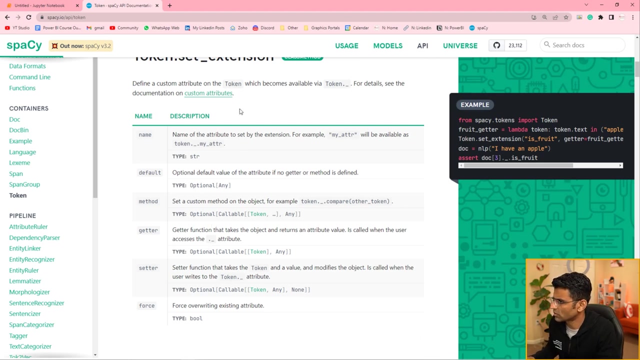 like URL, like number, so many other methods. okay, so you can check all those in a spacey documentation. how do I see spacey documentation? Google is your friend. spacey token attributes- okay, so I think, attributes- you can just Google and find it out. okay, I don't know, I don't know how to get to it. 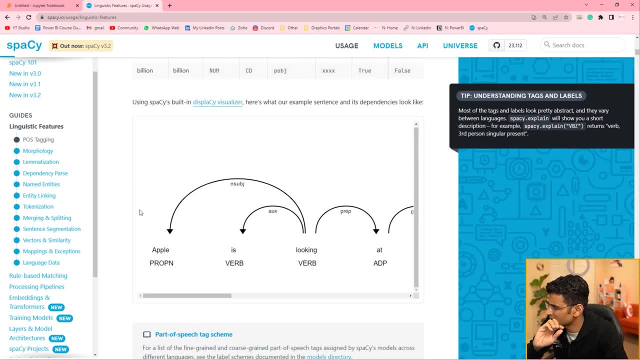 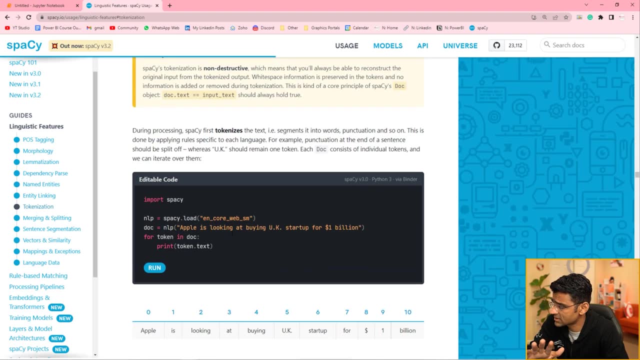 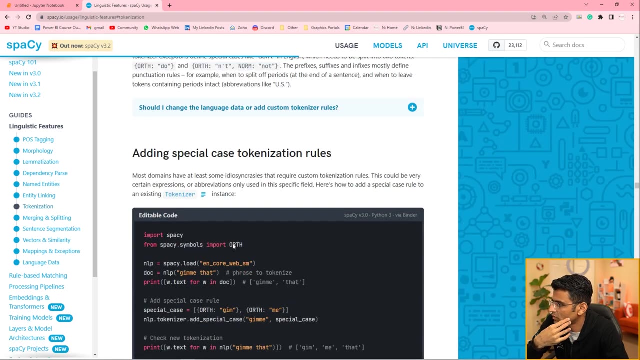 but you will find it out in in some documentation spaces. documentation, by the way, is really good. I really like that and see they have given a very good article. by the way, I highly suggest you read the article. you will see this is a chart that I use in my presentation. thanks, spacey folks. 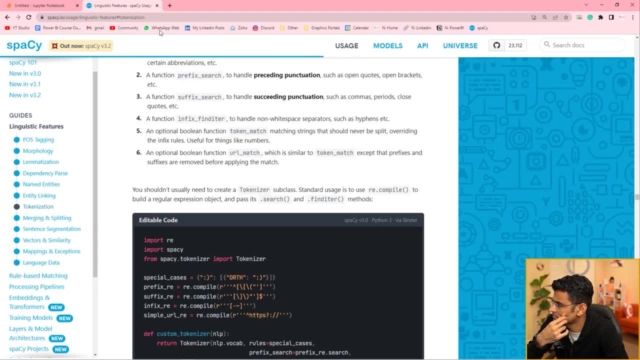 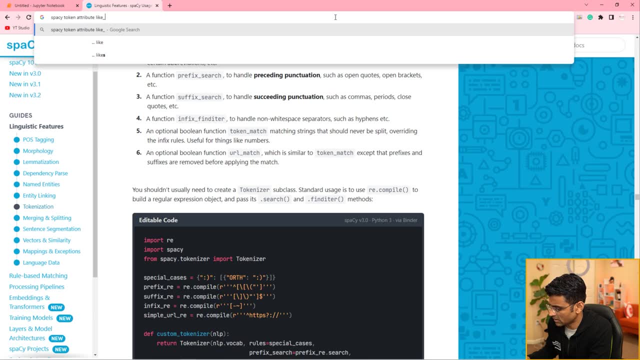 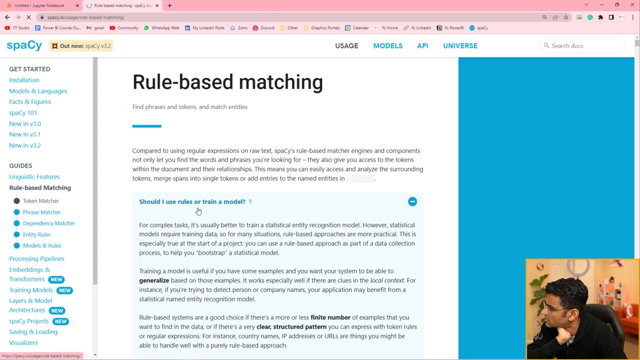 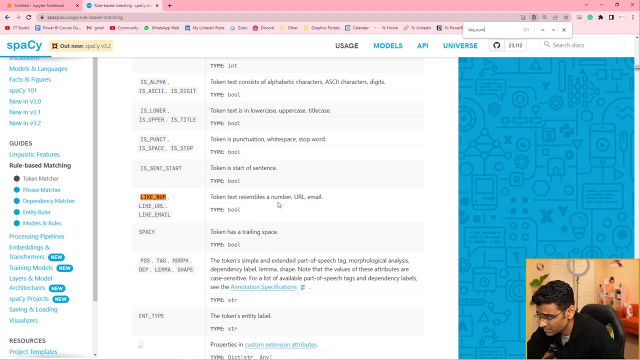 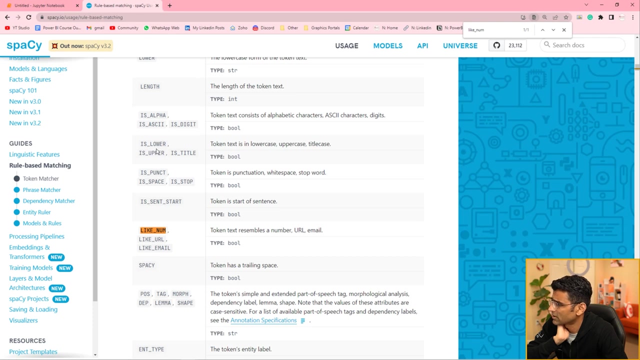 um, you can do spacey token attribute like number. see, these are all the um. these are all the all those tokens that we have. um, these are all the all those tokens that we have. okay, you have is alpha. is you have all of those? okay, correct? now let's move on to the next agenda. 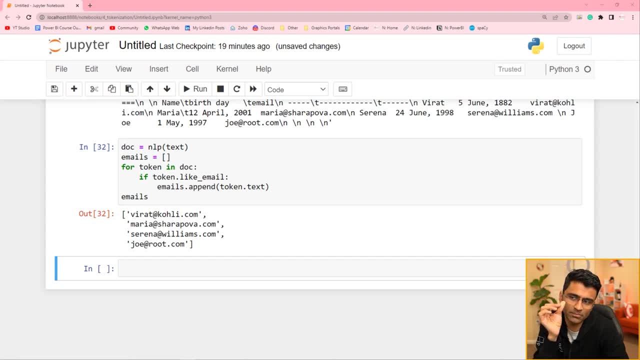 now we will try a model in a different language. so hindi is my, is the language of my country, india, so i will use hindi and the hindus code. we saw right, it is hi and i will create you know some something. i will take some sentence in hindi. 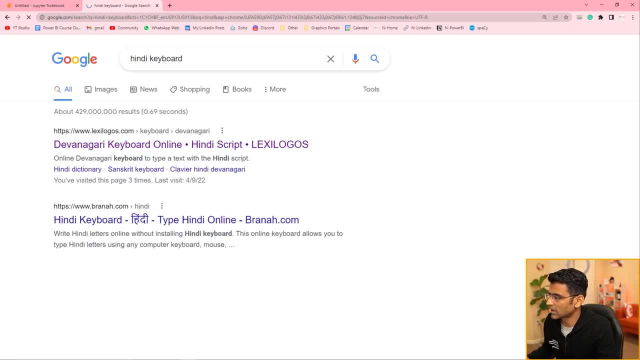 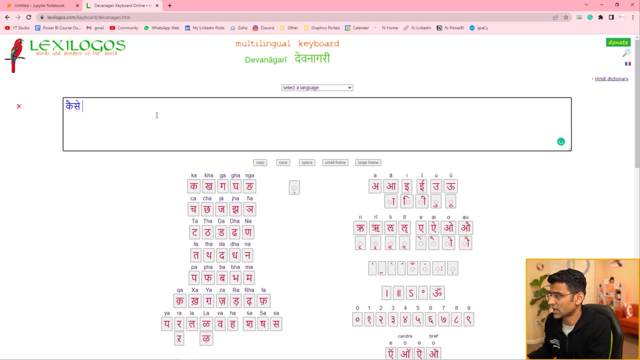 by the way, you can type in like hindi keyboard, and you can type it in hindi even with your english keyboard. you can say: see, this is like you can type it in hindi, and you can just say control c and control v. so, similarly, i typed something and i am. 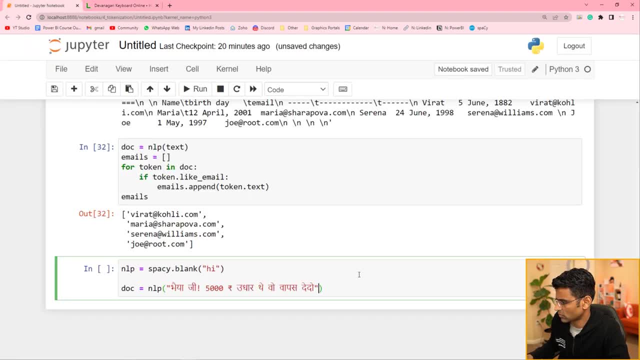 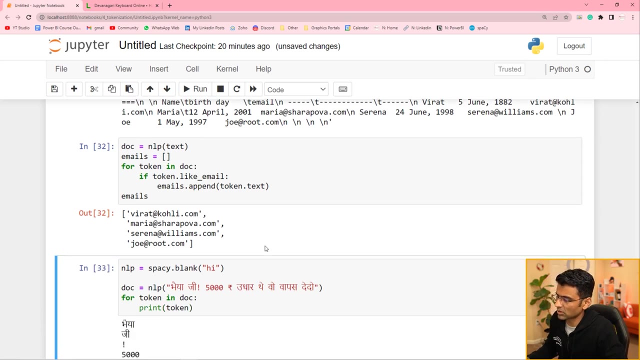 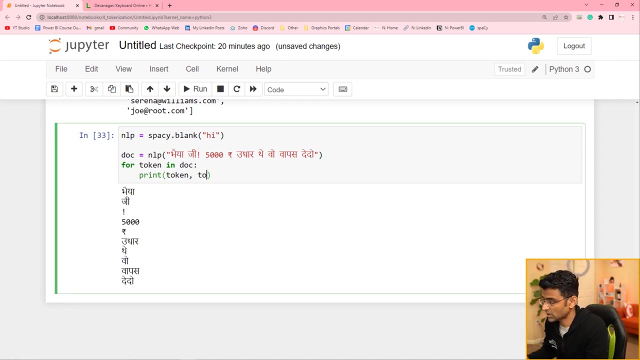 doing control C, control V, okay, saying like he's borrowed money from someone and he's asking to return them, and you will again do the same thing. just print all the tokens. and you see that it is printing all the tokens. not only that, along with the token you can print some of that to it, let's say, is currency and 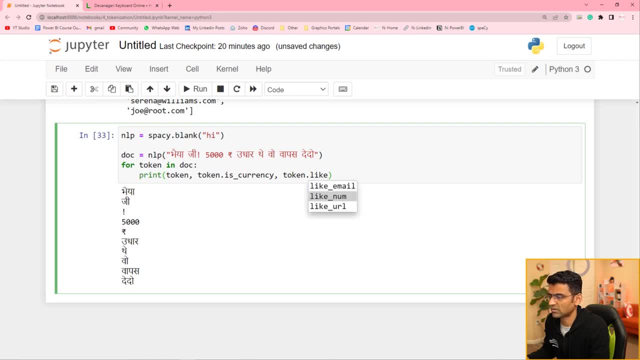 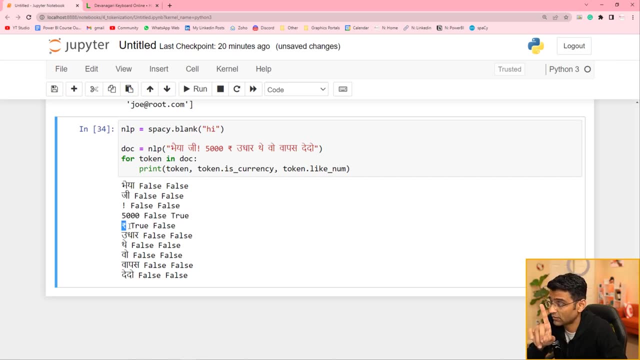 token dot like number right. so when you print that, see, for 5000, currency is false but number is true. and for the rupee sign, this is a rupee sign. a rupee sign it will say: is currency, yes, it is currency. so you take any language model. 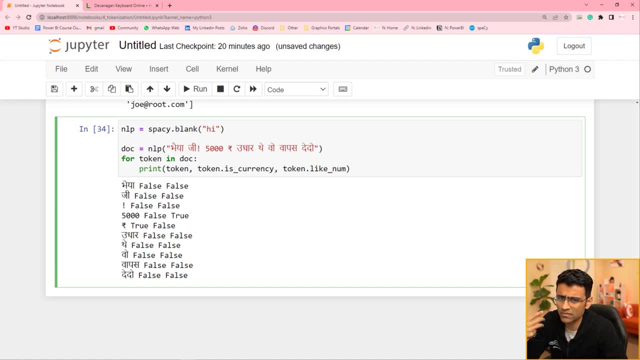 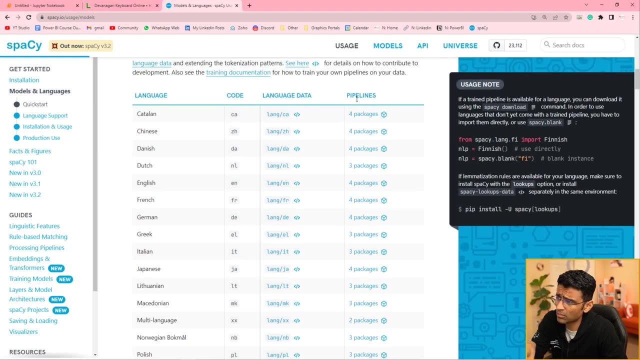 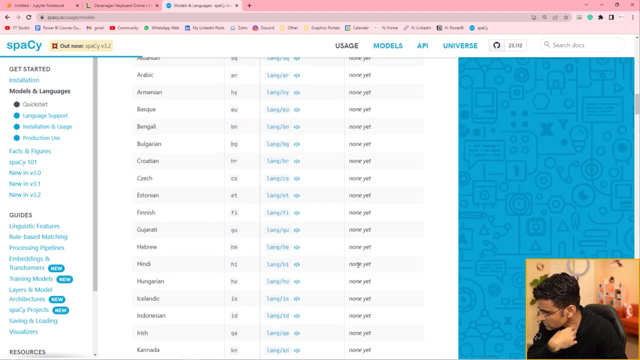 it is. it is having knowledge of these basic rules. now, if you look at this documentation, there is this column called pipeline and only few languages have these pipelines, but the other languages says none yet. see, Hindi says none yet. and what is that pipeline will cover later? okay, let's let's move on to the new, new. 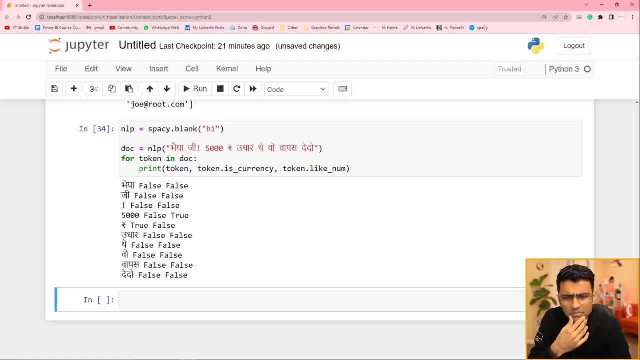 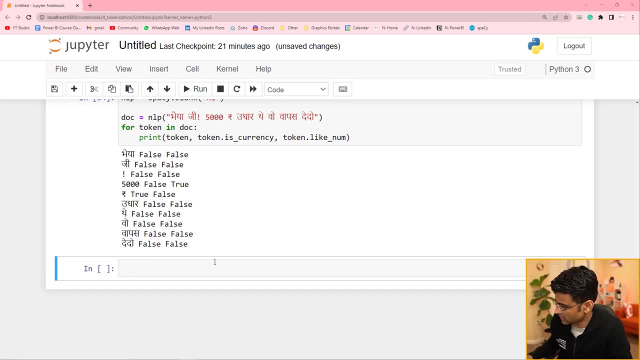 topic. so now, sometimes you want to customize your tokenizer, for example I. you have a sentence like this: can you say for? and, by the way, instead of you for token in token sprint I will try to grab everything in a in an array, so I will say token. you know list comprehension right, so list. 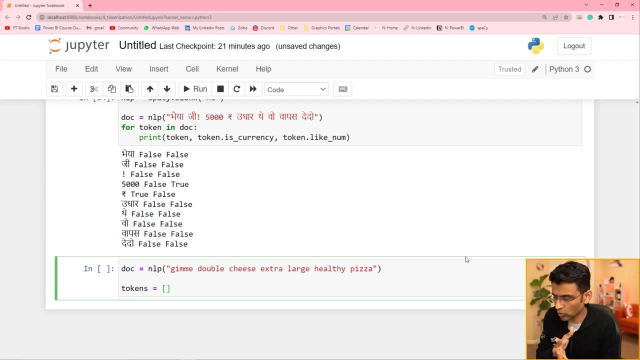 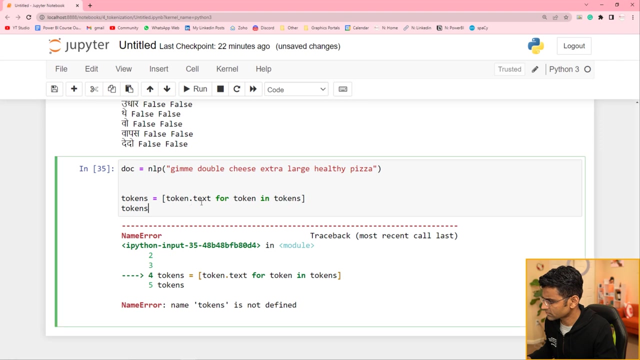 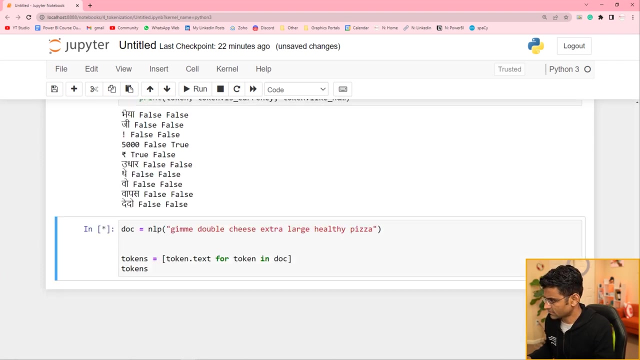 comprehension is a easy way to write for loop. so instead of writing for tokens, do something. I can move this thing here in a for loop and whatever you want to do, you can put that thing here. so when you do that, you get all these tokens. now you're not happy with the default behavior of spacey here because 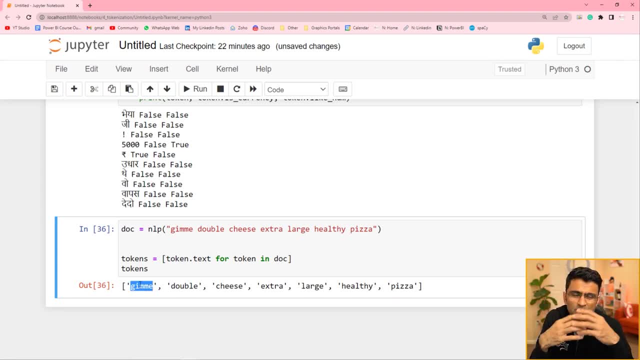 see, i use abbreviation when you use slang and specific norms of any language. that's when you realize the need of customizing spacey. so you get all these tokens. now you're not happy with the default behavior of spacey here, because give me is actually two words, give me, you want two separate tokens. so what you can do. 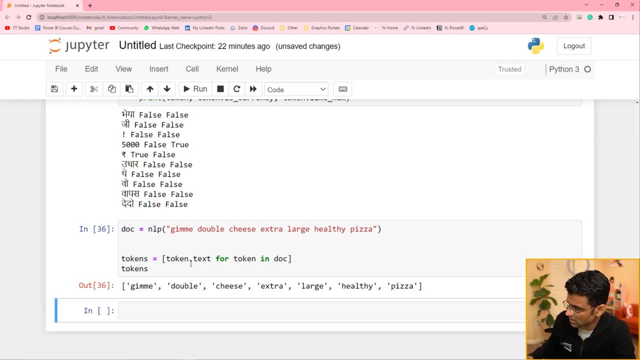 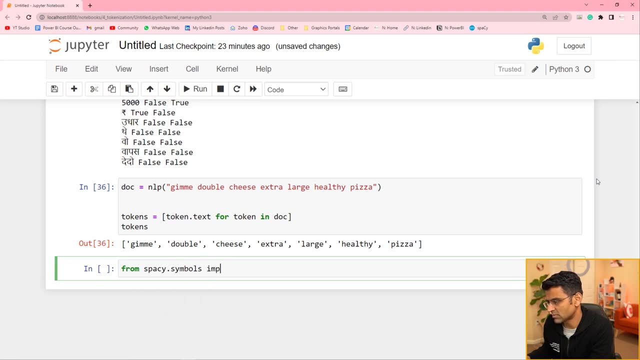 is. you can customize spacey here. by doing this, you can say: from spacey dot symbol import, or. and then you can say nlp dot tokenizer. you know we have the nlp object and you can say add space. so i'm, i'm adding a space. 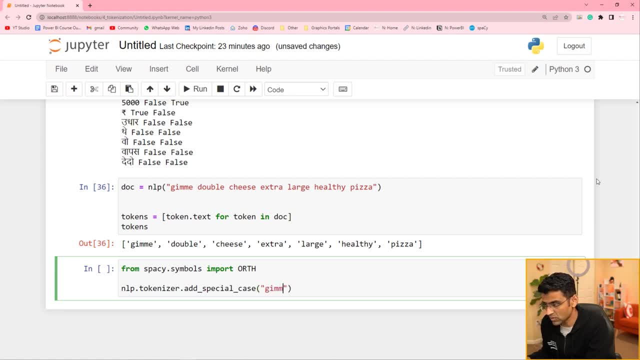 is okay. where i want to customize, give me into into what. so i want to use odd game. so you want to customize this to you and me, correct? so this don't worry about syntax too much. maybe you look into oz and other symbols we have available here. so i'm just going to 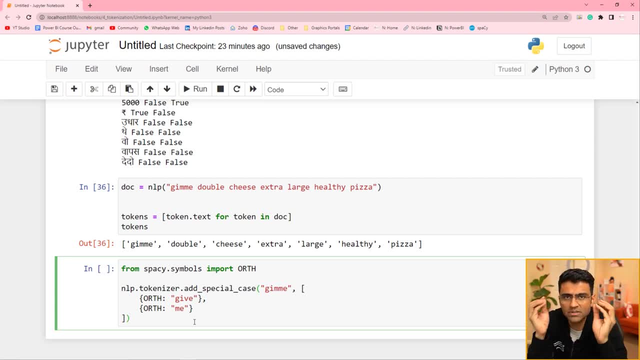 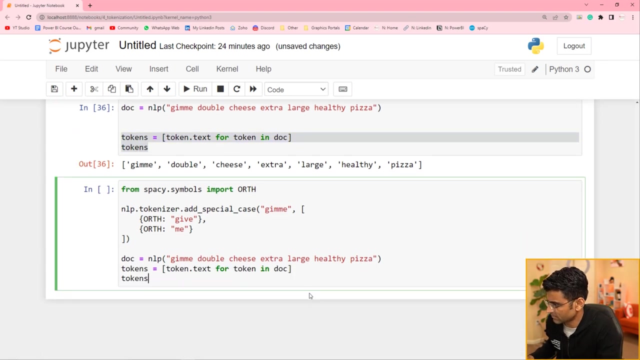 in later. but this is a simple way of customizing spaces behavior, where I'm saying: whenever I asked you to tokenize, give me just. give me two tokens instead of just one, give me token, okay, and then I will create a dark element and I'll do this same thing when I hit enter, if what it is saying is spatial cases are not. 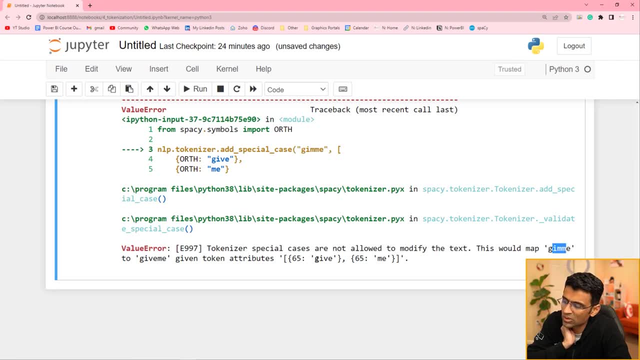 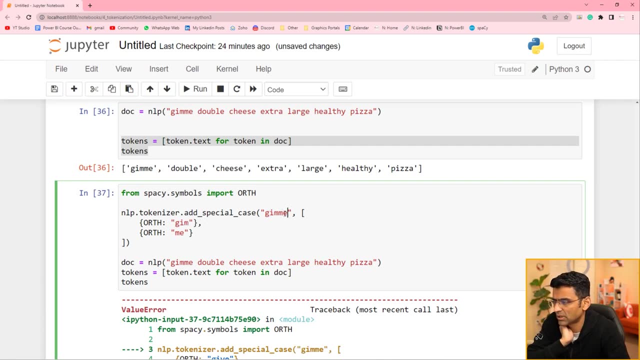 allowed to modify the text. so you can't do give me, you can't do give and me, but what you can do is you can do give me, so it's like give and me. so you can modify the actual word. you can split it, okay, and if you want to modify, will we have. 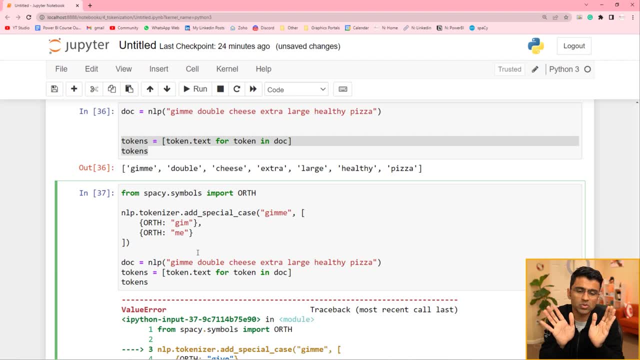 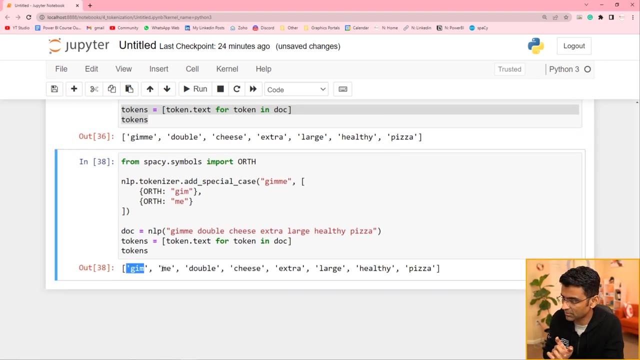 further processing steps. tokenization is just by. tokenizing is kind of a little dumb. it just splits the whole thing into segments. you don't want to change the actual text. that's not allowed. when I do this now, see, I get give and me as two different tokens. alright, so that was about adding. 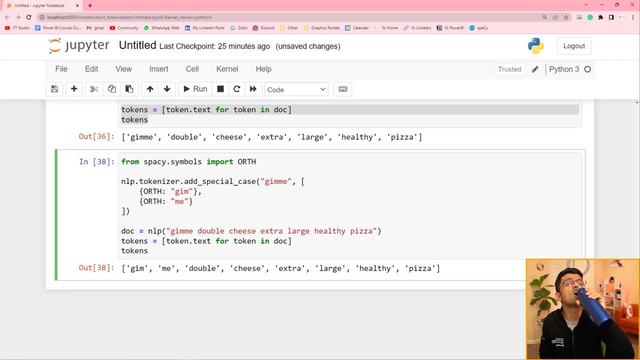 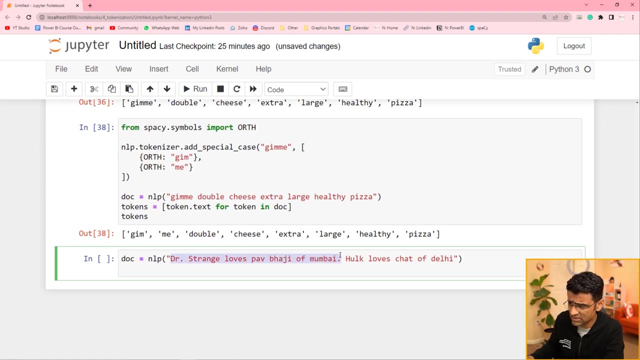 a spatial rule in tokenizer. now let's do you sentence tokenization. this is something we have looked into it before also, so I will not spend too much time and here I have two sentences: Hulk and strange. both are loving India trip, enjoying the food to rim. to tokenize this into sentences: 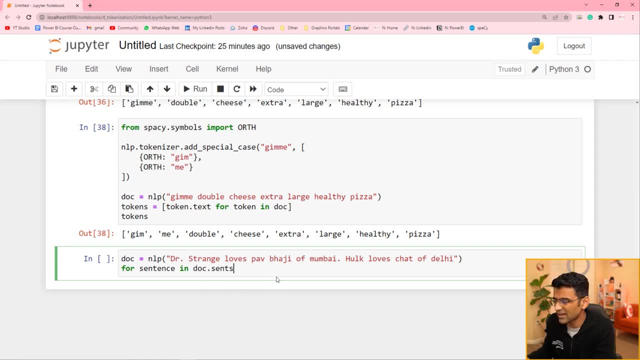 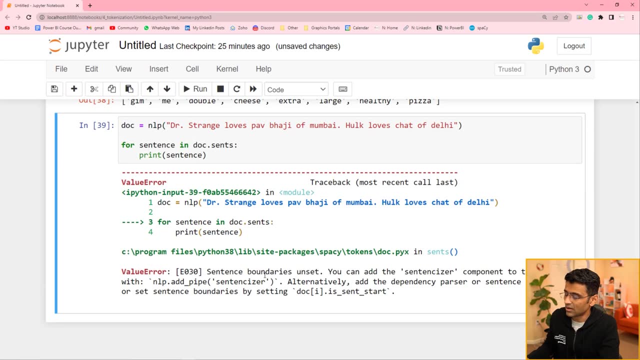 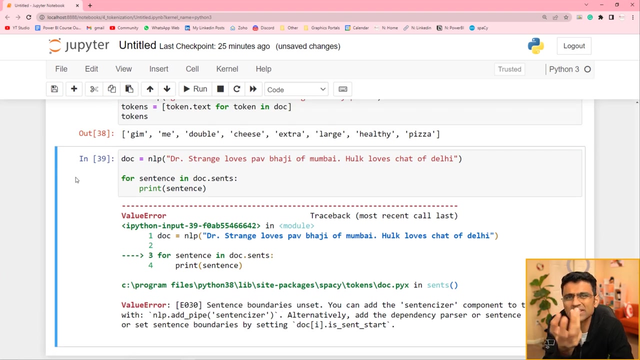 you can say for sentence in doc dot send senses sentence. isn't that obvious? hmm, this is not working. what is the error? let's read: so it is saying my NLP pipeline is kind of blank. that's what this Adam means. it's not saying that. so 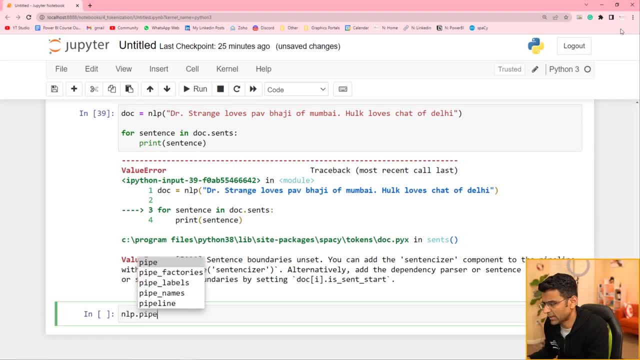 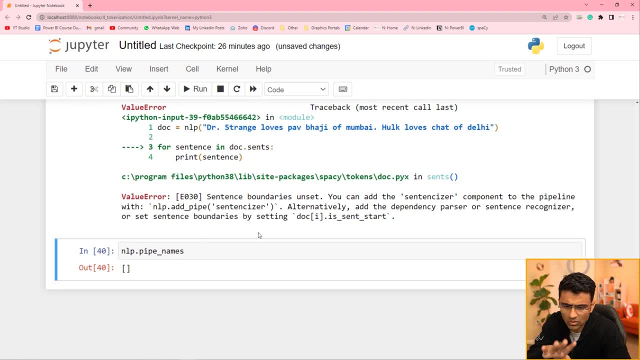 if you do NLP dot pipe pipe names, that pipeline is blank and what does that pipeline means? so what I can do is: here I can add NLP dot air pipe, because that's what it is asking me to do, and I'm adding a sentence sizer into it. and when I do that, see my pipe names, remember it. 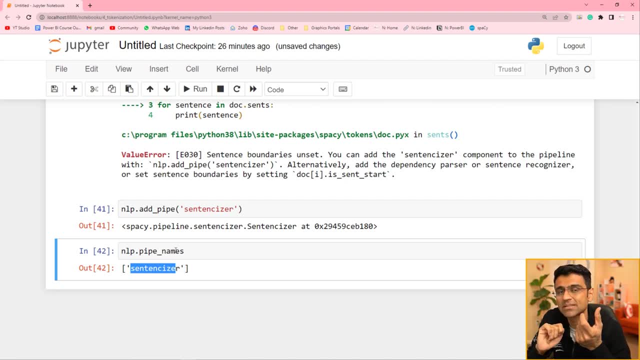 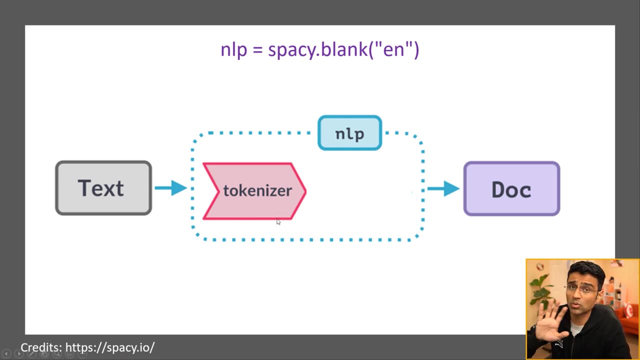 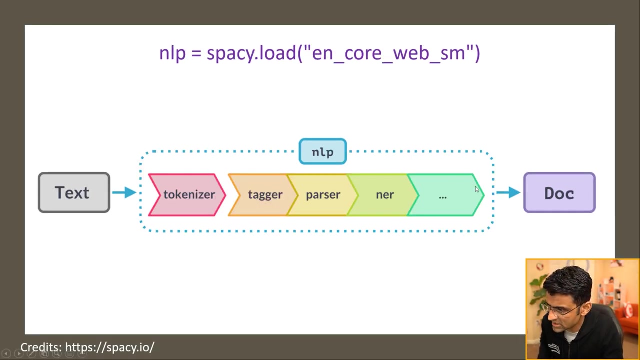 was empty. now my pipeline has this sentence: sizer component. so what I did essentially is this, if I can open my presentation: blank pipeline is like this: you only get tokenizer, you don't get any other component. but when you build a pipeline- see this, the second part, this whole thing- 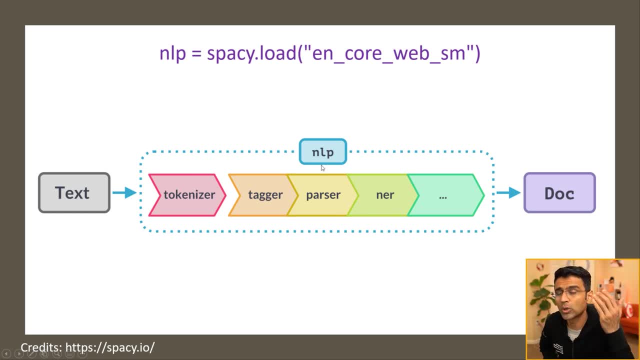 is called pipeline and it has different component- we will look into it later- like tagger, parser, name, entity recognizer. we'll see all those details, but the simple idea you want to learn today is: you have a blank pipeline when you do this. but when you do something like 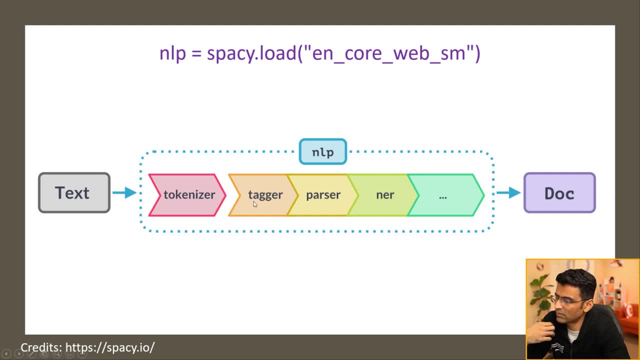 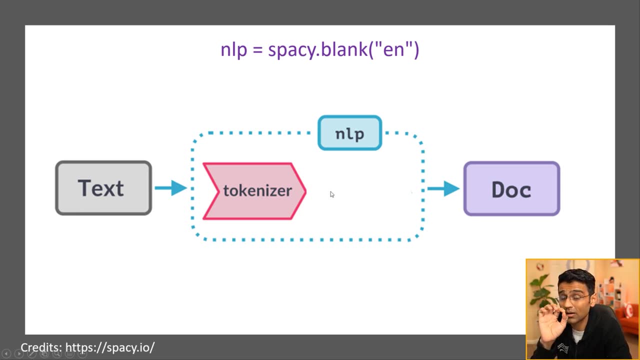 spacey dot load, you get full-fledged pipeline where you can have these components and and if you have a blank pipeline you can add a component in the pipeline manually. and that's what we did when we did spacey dot add pipe. here, after tokenizer component, we added a component for 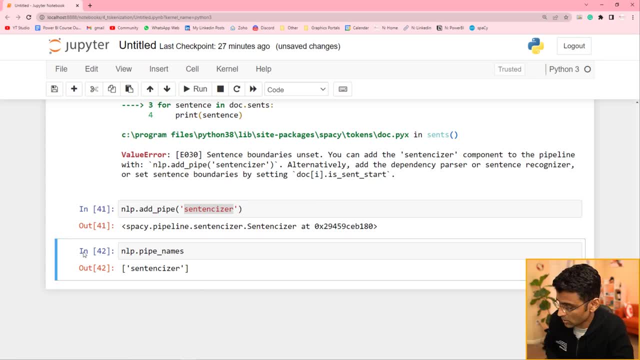 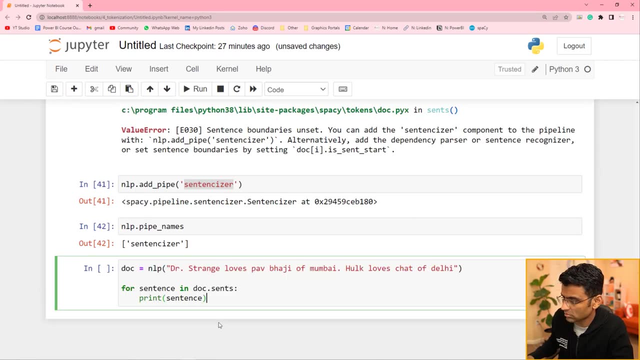 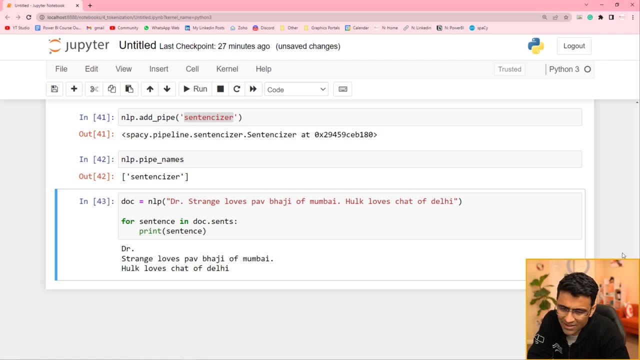 sentence. sizer, which means now this NLP object knows how to split the sentence into, how to split paragraph into sentences, and when you do that, see it is doing all this and it's kind of little strange because the component that I added is little dumb and it is splitting. see after dr, when it sees dot, it is splitting that into. 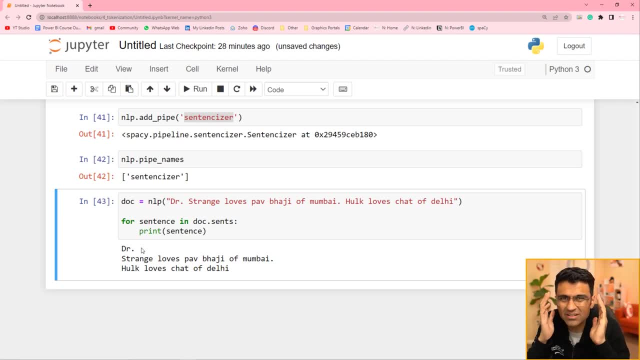 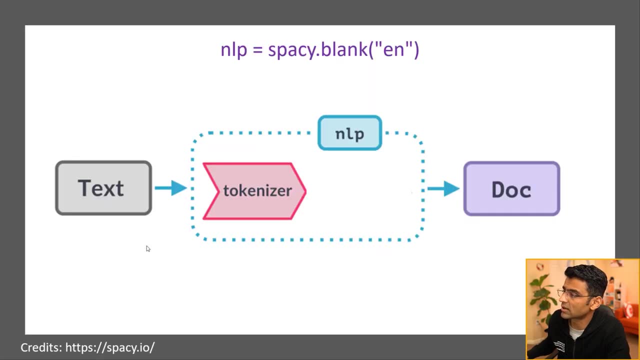 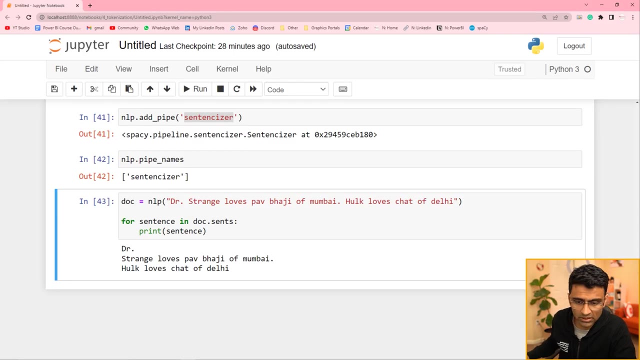 uh, it is thinking it's a separate sentence. so it still doesn't understand English language fully. and we'll see in the next video probably, that when we use pipeline like this, it will fix all those issues. so we'll look into those later, uh, in in the future chapter, in the future video. 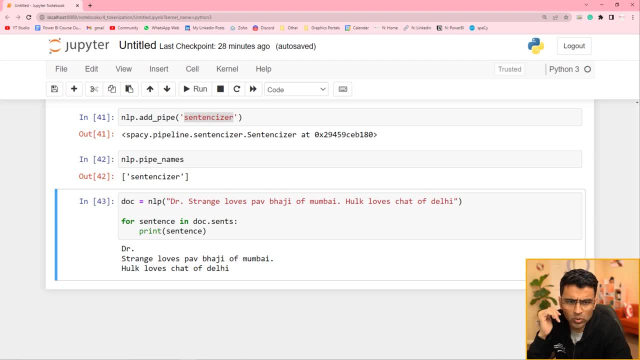 okay, so that's all I have for the tokenizer now. it's the most interesting part of this tutorial, which is an exercise. yes, it's like swimming. if you watch a swimming video, you're not much better than this, so hope you enjoyed it by taking advantage of this video. 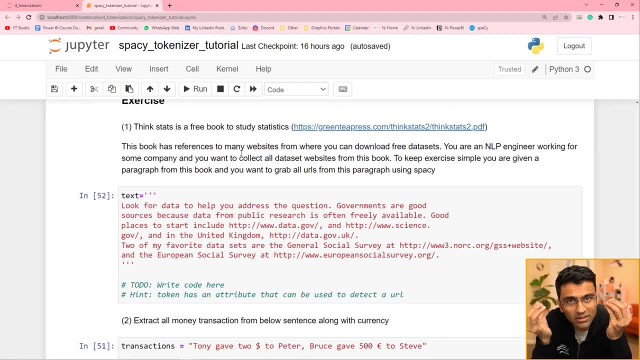 video. you're not going to learn swimming. you want to make a career in nlp. you want to earn big money- by the way, nlp engineers make a lot of money. okay, if you want to achieve a heights in your career success, you have to work hard. for that reason, i'm giving you this exercise where 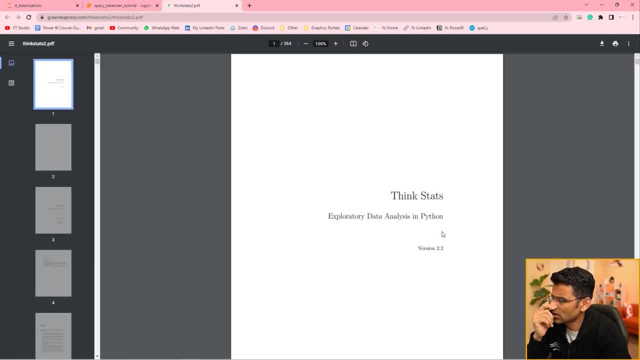 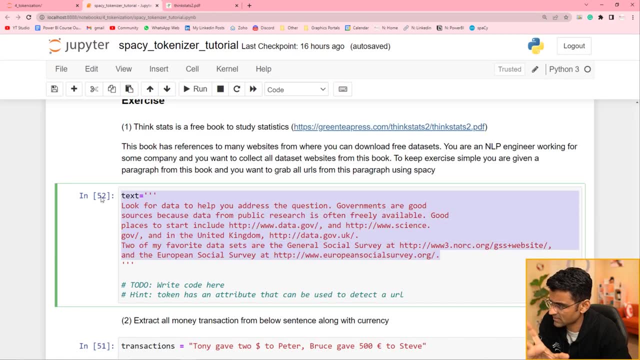 you might know about this thing- stats book. so this is a nice book, free book for learning statistics, and a paragraph of this book is this: i just took some paragraph from that book. okay, that contains couple of urls for free data set website: see free data set website is something. 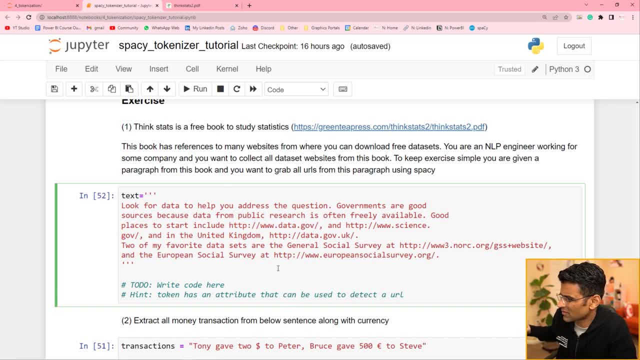 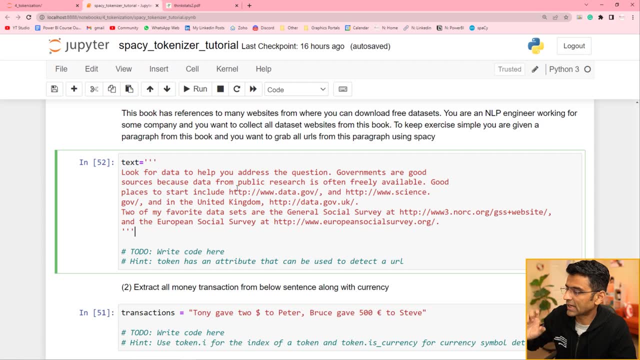 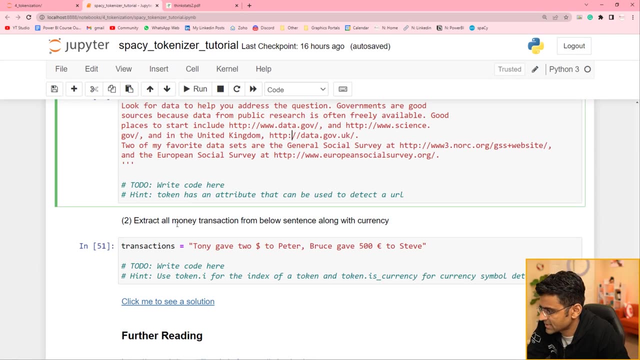 that you need as an nlp engineer working for a company. so i want you to write a code here that can process this text paragraph and grab all these data urls. see one, two, three, four, five. and the second exercise is you have to extract all the transaction money, which is the 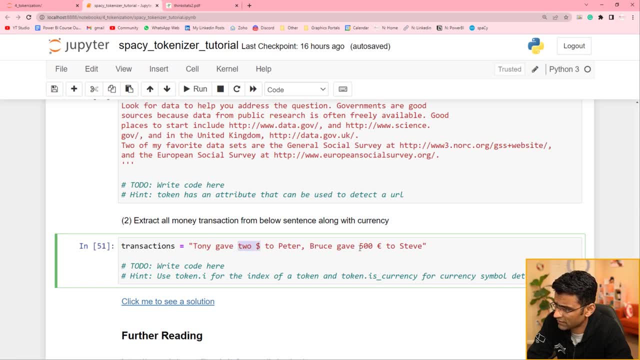 answer will be two dollar and five hundred euro. so the answer of this would be two hundred dollar and five hundred euro, and you have to, you know, write some code to extract that. this sex will require little thinking. I have a solution here and it is very tempting to click on the solution, but I know you all. 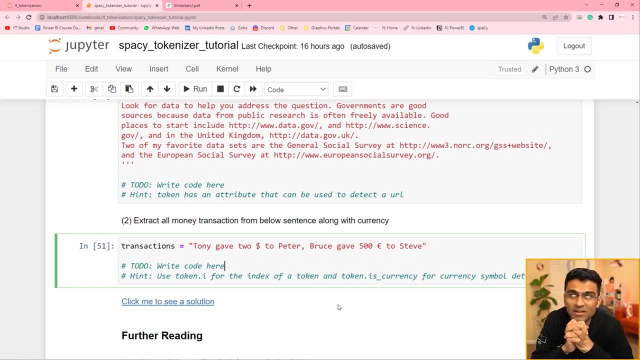 are brilliant- not brilliant, but sincere students. so I'm pretty sure you will not click on this solution link. you will work on on it on your own. and if you click on it before without trying it, look, I have a magic embedded here. so when you apply for NLP engineer job, you know you will probably not get an.